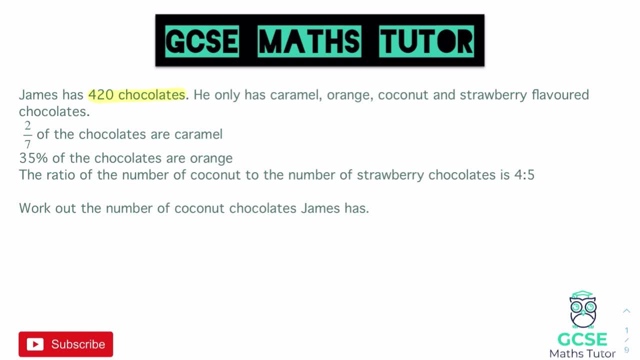 is four to five, and it wants us to work out the number of coconut chocolates that James has. So let's have a look. We've got two sevenths that are caramel, and we've got the next bit of information there that tells us that 35% are orange, and then it goes on to tell us that coconut 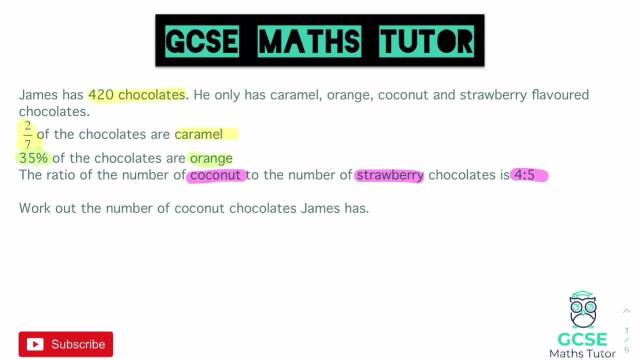 to strawberry is four to five. So if we start with the first piece of information here, and that's the two sevenths are caramel. So if we start with the first piece of information here, and that's, the two, sevenths are caramel. So to break this down, we'll start working out one of those pieces of information. 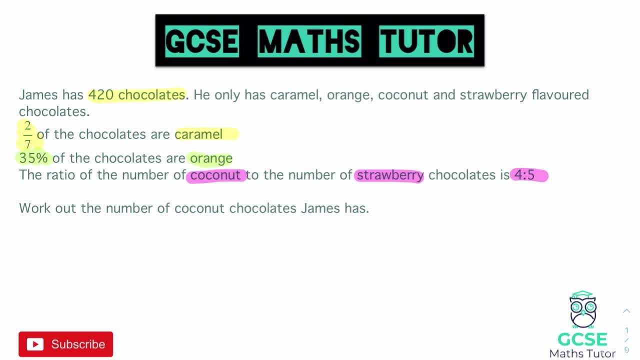 So to work out two sevenths of a number, obviously you need to know how to work out a fraction of an amount. here We're first going to work out one seventh and to get one seventh we're going to divide 420 by seven. So obviously, if you have a calculator, this sort of question is relatively 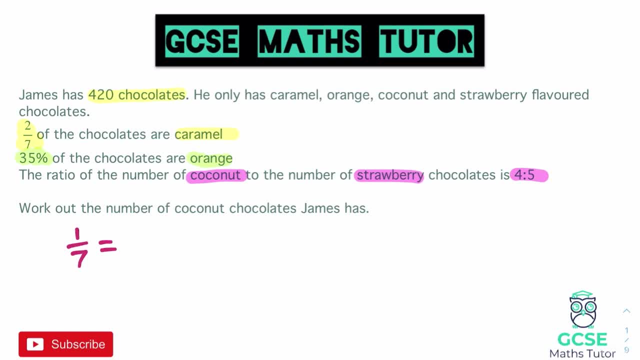 simple in terms of the calculations. but if you don't, you're just going to have to do a little bit of bus stop method to the side and working out seven into 420. So seven goes into 42, six times, and then seven doesn't go into zero obviously. So we have 60 there. So one seventh. 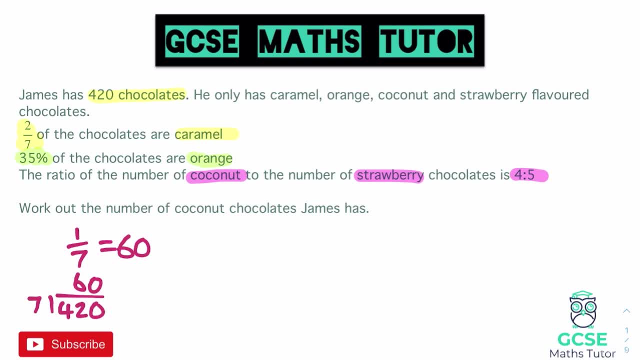 would be 60 chocolates, and obviously always leave your working out to the side. I'm going to get rid of that because we need the space, but obviously always leave your working out. Now we want two sevenths, So we'll double that. So two sevenths would be 120.. And then we've got our first piece. 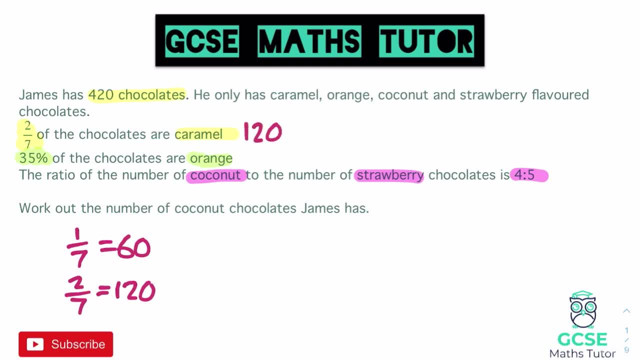 of information We've got, there are 120 caramel chocolates. Now we can move on to the chocolate chocolates that are orange. So again, if we get rid of this and we'll just focus on the working out- in fact we'll just leave that there for the moment- We'll go with working out the 35% first. 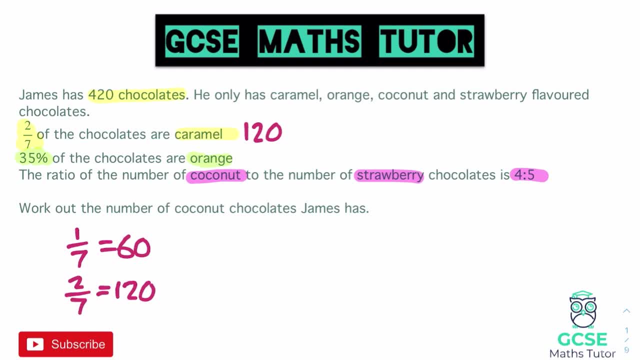 So to get 35% again, if we'll assume that we don't have a calculator for this, we'll work out 10% and use our non-calculator method. So 10% is going to be 42 and 5%, which is half of that, is going to. 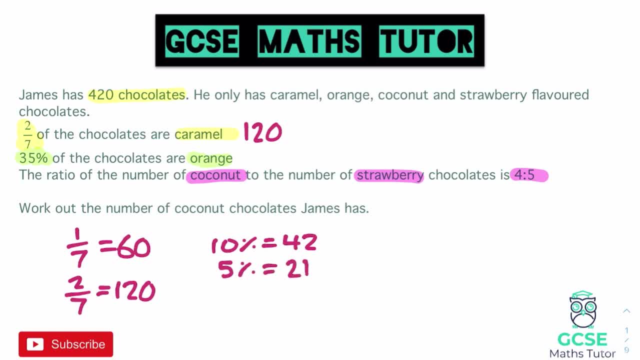 be 21.. So in order to get 35%, we're going to want three of the 42s. That takes up to 30%, And then we'll add the 21.. So completely up to you how you do that. You can either multiply that. 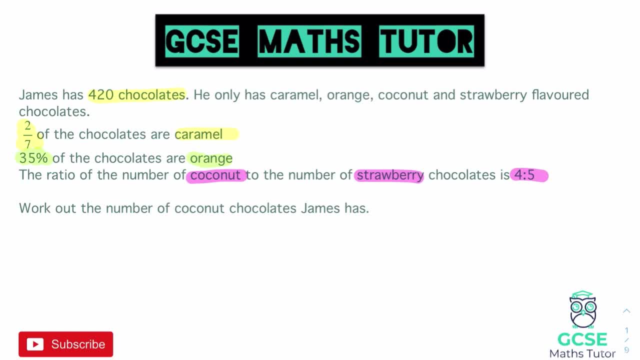 to strawberry is four to five. So if we start with the first piece of information here, and that's the two sevenths are caramel. So if we start with the first piece of information here, and that's, the two, sevenths are caramel. So to break this down, we'll start working out one of those pieces of information. 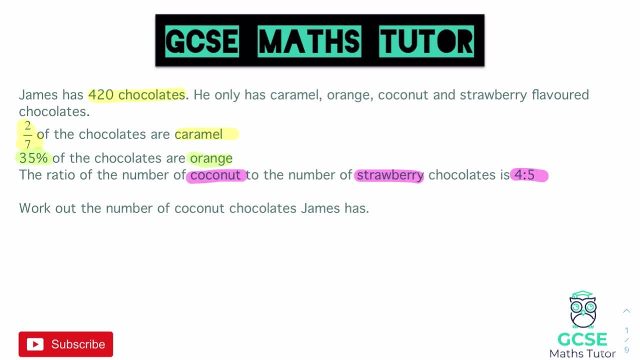 So to work out 2 sevenths of a number, obviously you need to know how to work out a fraction of an amount. here we're first going to work out 1 seventh, And to get 1 seventh we're going to divide 420 by 7.. 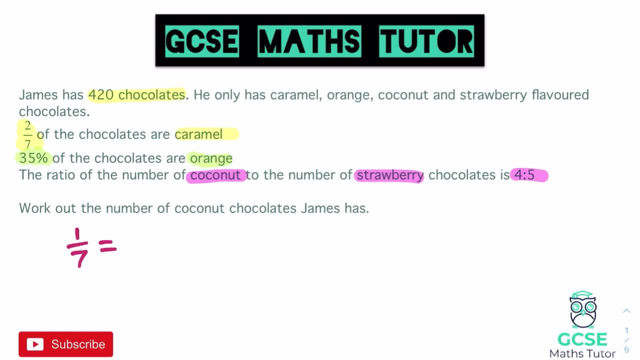 So obviously, if you have a calculator, this sort of question is relatively simple in terms of the calculations. but if you don't, you're just going to have to do a little bit of bus stop method to the side and working out 7 into 420. 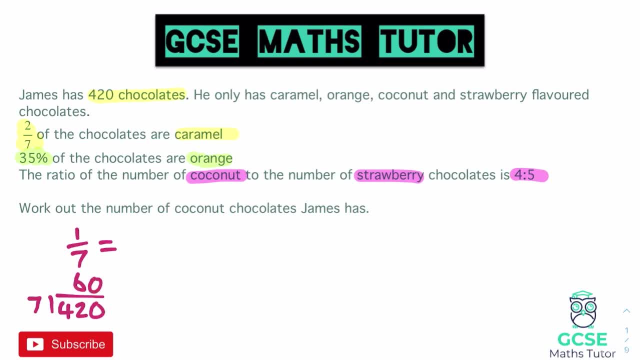 So 7 goes into 42 six times and then 7 doesn't go into 0 obviously. so we have 60 there. So 1 seventh would be 60 chocolates, And obviously always leave your working out to the side- I'm going to get rid of that because we need the space- but obviously always leave your. 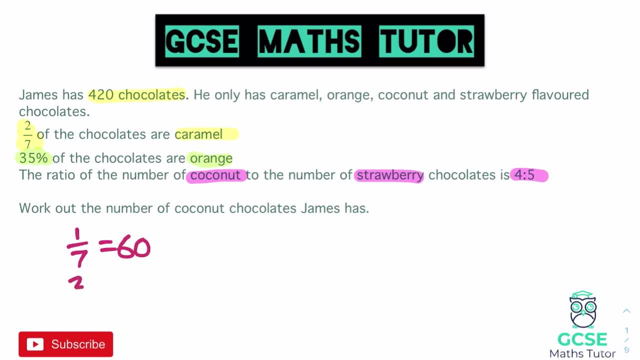 working out. Now we want 2 sevenths, so we'll double that. So 2 sevenths would be 120.. And then we've got our first piece of information We've got: there are 120 caramel chocolates. Okay, Now we can move on to the chocolates that are orange. 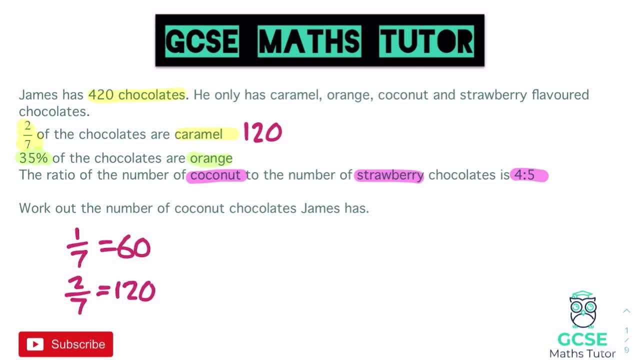 So, again, if we get rid of this and we'll just focus on the working out- in fact we'll just leave that there for the moment- we'll go with working out the 35% first, So to get 35% again. if we'll assume that we don't have a calculator for this, we'll 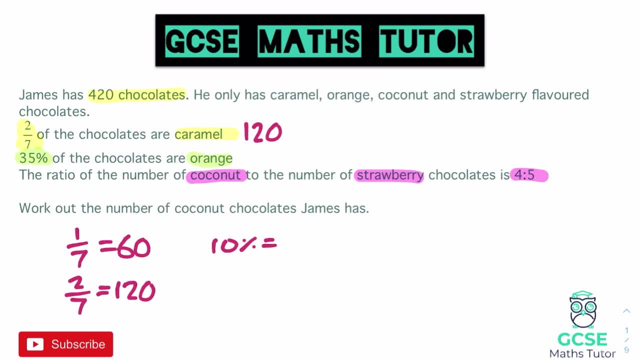 work out 10% and use our non-calculator method. So 10% is going to be 42, and 5%, which is half of that, is going to be 21.. So, in order to get 35%, we're going to want 3 of the 42s. 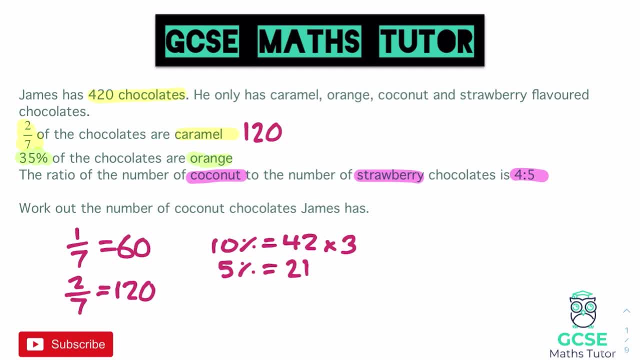 That takes up to 30%, and then we'll add the 21. So completely up to you how you do that. You can either multiply that by 3 and add 21,, or just to the side again, always showing your working out. 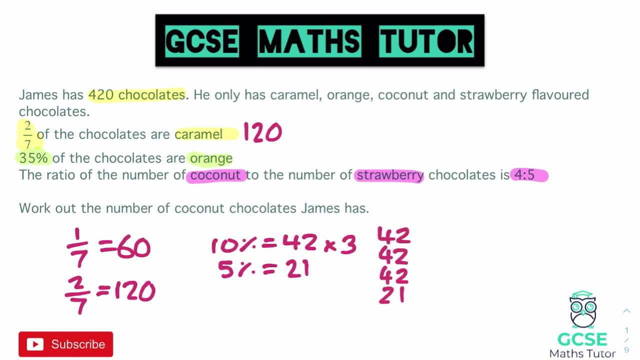 We could just add 3 of them together and then add the 21 and add that all up. We get 7 and 4,, 8,, 12,, 14, so we get 147. And then let's add that up here next to our information, and that is 147 orange chocolates. 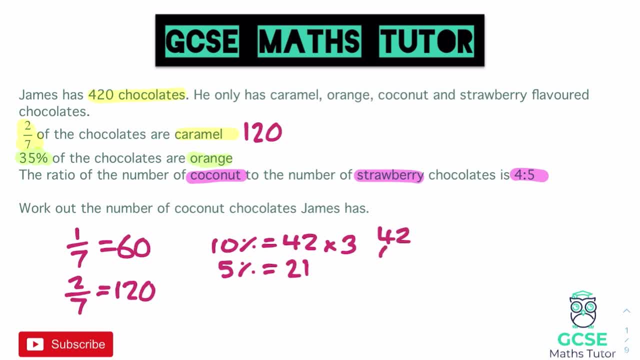 by three and add 21, or just to the side Again, always showing your working out- We could just add three of them together and then add the 21 and add that all up. We get seven and four, eight, 12,, 14. So we get 147. And then let's add that up here next to our information, And that is 147. 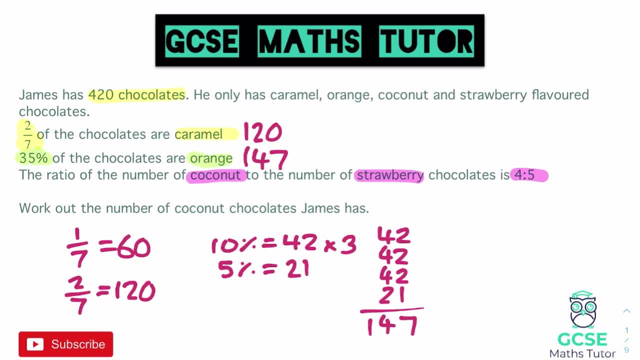 orange chocolates. Now we've got one last piece of information and we're going to get rid of all of this and just focus on that for now. So this last piece of information here tells us that the number of coconut to the number of strawberry is in the ratio four to five, And that is going to be for the remaining chocolates after. 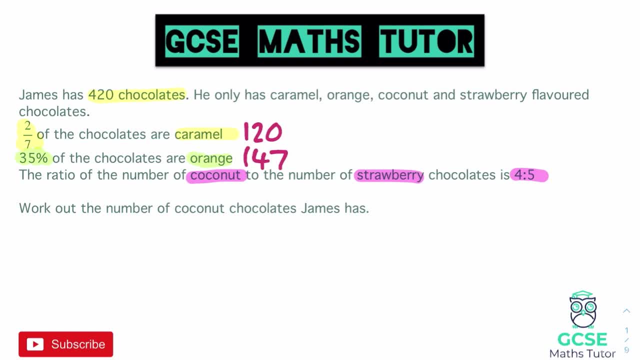 we get rid of the caramel and the orange, Okay. So we need to actually work out how many are left just for those. So if we add together the 120 and the 147, that adds up to a total of 267.. Now we need to take that away from the total, And we know that the total was 420. 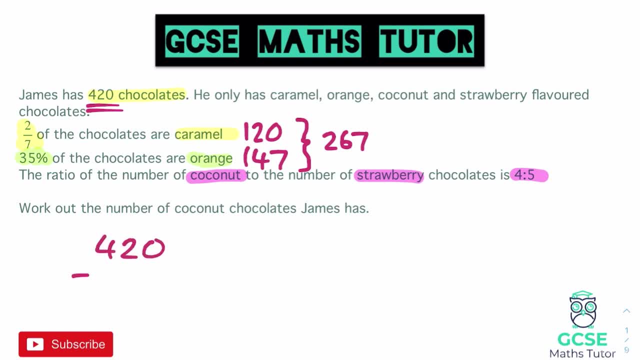 So 420, and we'll take away 267.. And again, without a calculator, we're going to have to do a bit of work here. Seven from 10 is three. We're going to have to carry again Six from 11. 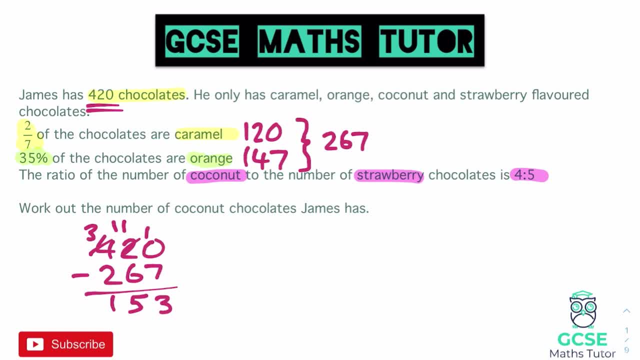 is five, and two from three is one. So that leaves us with 153 chocolates that are going to be coconut or strawberry. So we're going to write this as a ratio, So coconut to strawberry, and that is four to five. like that one, there's an s and a five next to each other. they look so similar. so we've got 153. 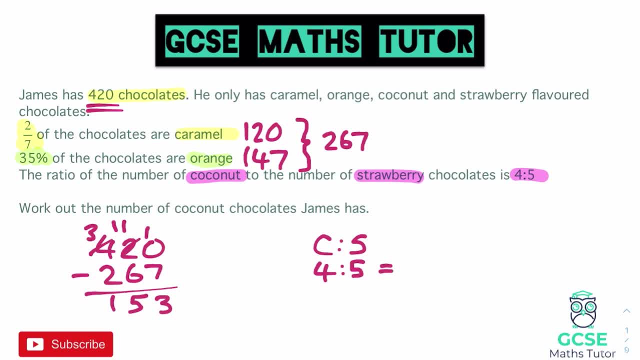 that we're going to share in that ratio. so four and five gives us nine parts in total and again, this is sharing in a ratio. so again, if you need any reminders on how to share in a ratio, i'll put the link for this video in the description so you can go have a look at sharing in a ratio, if you. 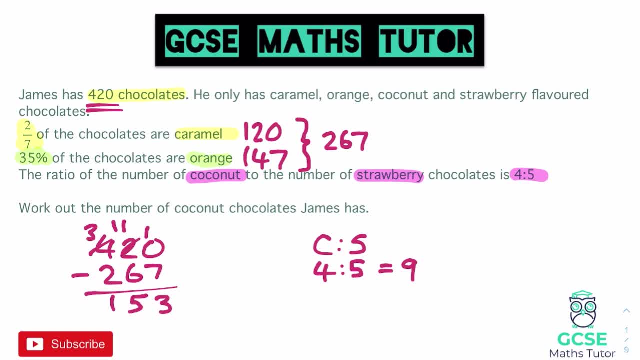 need to, but let's share this 153. so we've got 153 that we need to divide by nine, and again, if we're not doing this with a calculator, we'll divide that by nine and see what we get. so nine goes into 15 once, with a remainder of six, and then nine goes into 63 seven times. so that leaves us with 17. 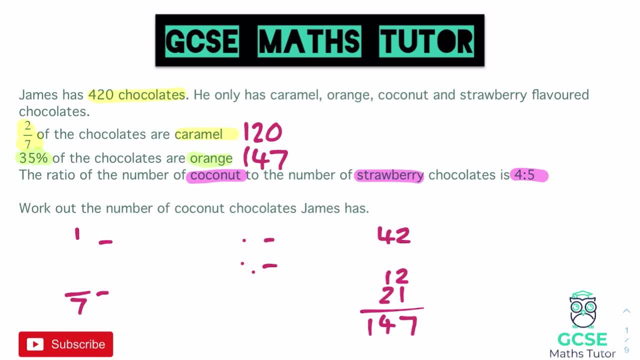 Now we've got one last piece of information And we're going to get rid of all of this and just focus on that for now. So this last piece of information here tells us that the number of coconut to the number of strawberry is, in the ratio 4 to 5.. 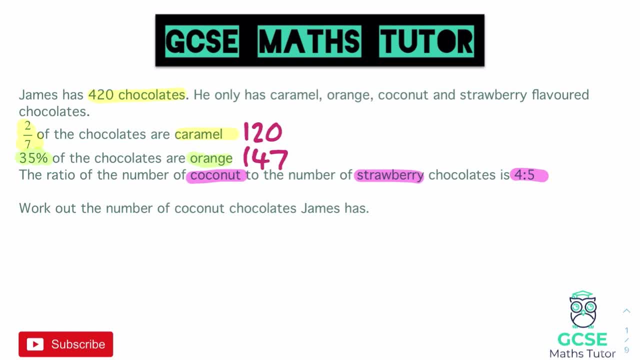 And that is going to be for the remaining chocolates after we get rid of the caramel and the orange. Okay, so we need to actually work out how many are left just for those. So if we add together the 120 and the 147,, that adds up to a total of 267. 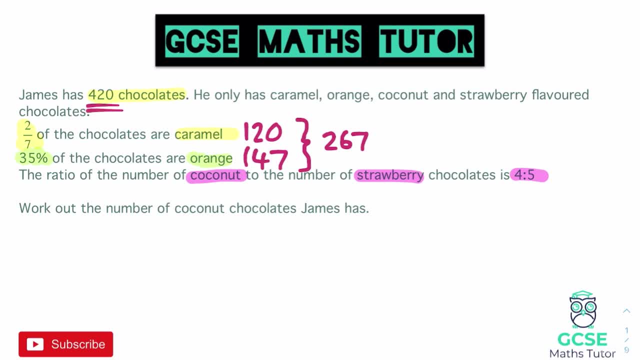 Now we need to take that away from the total, So we're going to add that up here next to our information, And we know that the total was 420.. So 420, and we'll take away 267. And again, without a calculator, we're going to have to do a bit of work here. 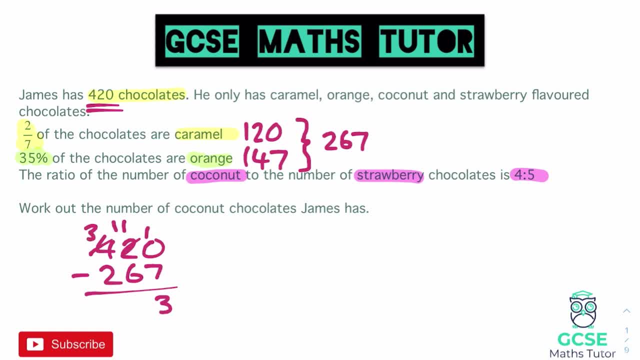 Seven from 10 is 3.. We're going to have to carry again. Six from 11 is 5, and two from 3 is 1.. So that leaves us with 153 chocolates that are going to be coconut or strawberry. 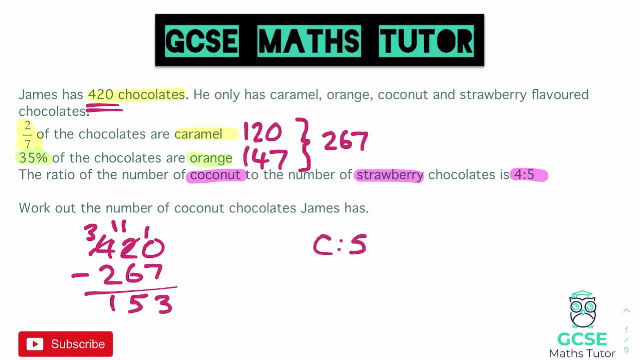 So we're going to write this as a ratio. So coconut to strawberry, That is 4 to 5.. I don't always dislike that when there's an S and a 5 next to each other, They look so similar. So we've got 153 that we're going to share in that ratio. 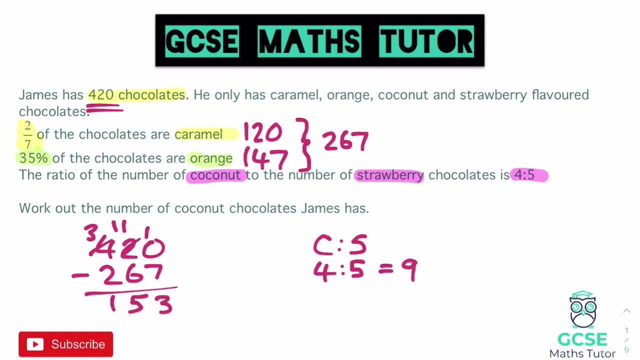 So 4 and 5 gives us 9 parts in total And again this is sharing in a ratio. So again, if you need any reminders on how to share in a ratio, I'll put the link for this video in the description so you can go have a look at sharing in a ratio if you need. 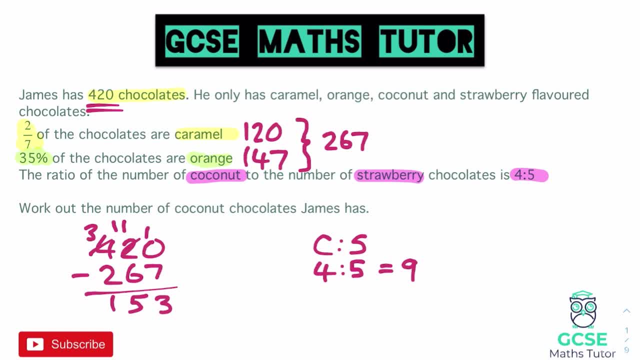 to, But let's share this 153.. So we've got 153 that we need to divide by 9.. If we're not doing this with a calculator, we'll divide that by 9 and see what we get. So 9 goes into 15 once, with a remainder of 6, and then 9 goes into 63, seven times. 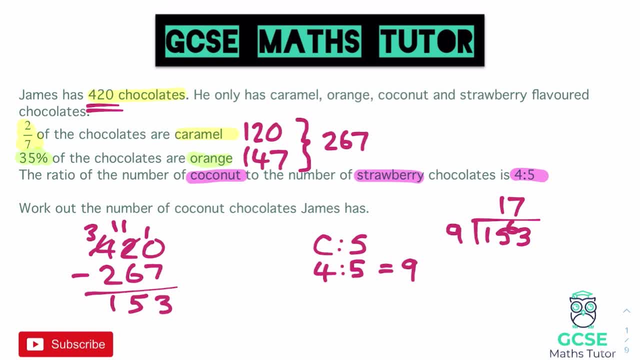 So that leaves us with 17. So for this one part is equal to 17.. So with our ratio, in order to turn these into the actual amount of sweets, we need to multiply them both by 17. So again we can do 4 times 17.. 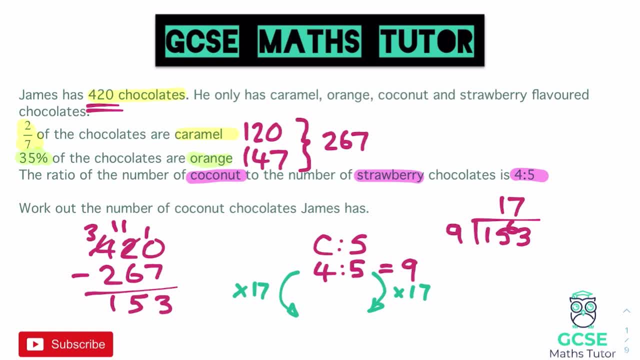 And again, you can just multiply that to the side. We'll add them up using column addition, but that is going to be equal 68. And if you do 5 times 17,, that's going to equal 85. So there we go. 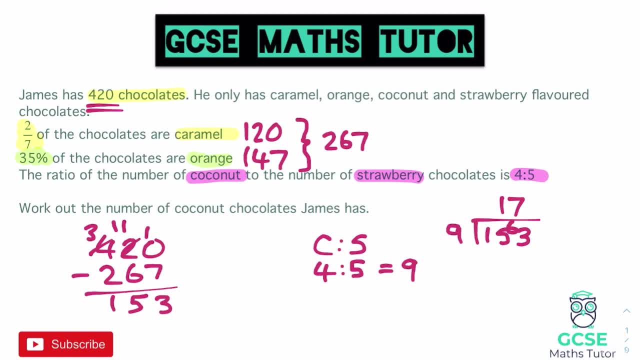 so for this one part is equal to 17. so with our ratio, in order to turn these into the actual amount of sweets, we need to multiply them both by 17. so again we can do 4 times 17 and again you can just multiply that to the side or add them up. 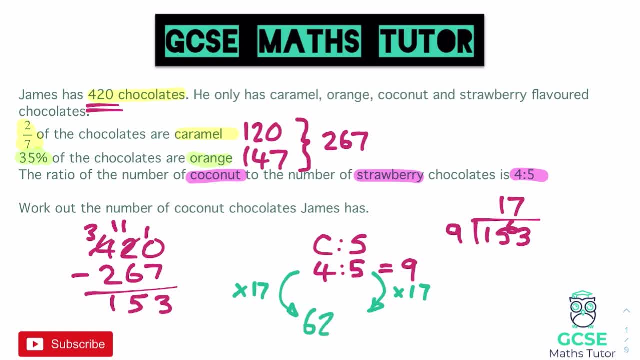 graphically, or you can just multiply that to the side or add them up stairs. we can apply them in column addition. then that is going to be equal 68. And if you do 5 times 17,, that's going to equal 85. So there we go. that is all of our amounts there. If we apply that. 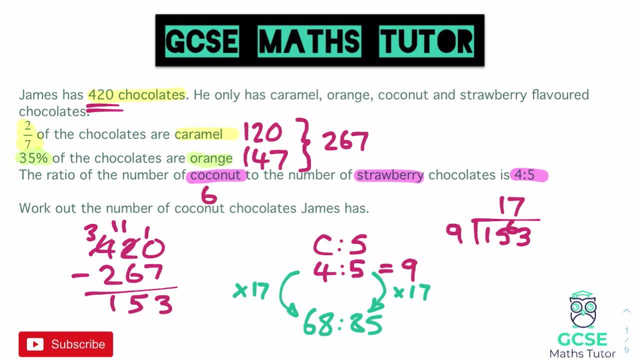 back to the question. underneath coconut there we've got 68, and underneath strawberry we have 85. Now the question here did only say: work out the number of coconut chocolates that James has. so for our final answer we would say 68,, as that was the amount of coconut. 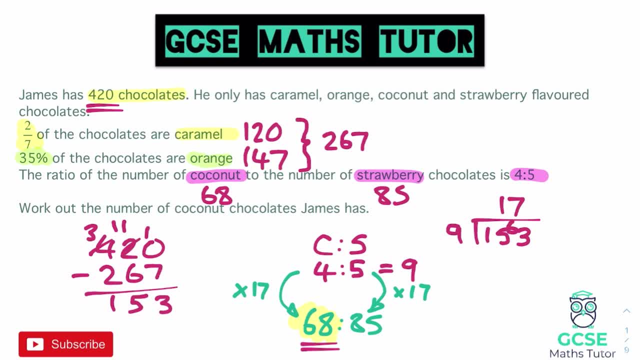 that we had after we worked out that ratio. So there we go. there was a lot going on in that question. you had to work out a fraction of an amount, a percentage of an amount, finding out what was left and then sharing that in a ratio. So a lot going on in this question. 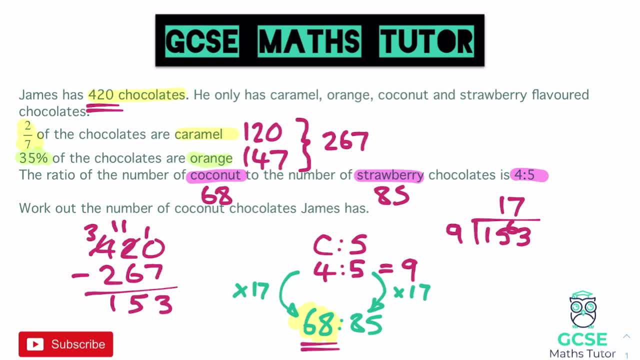 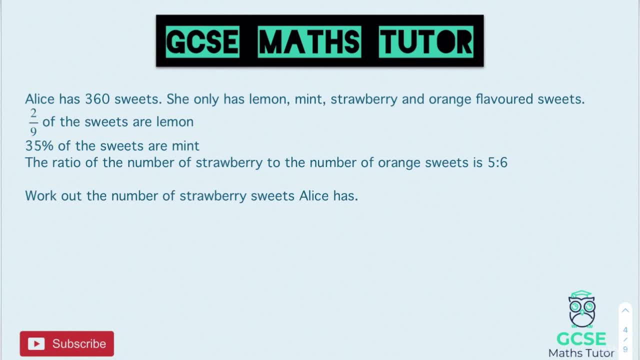 but I'm going to give you a question very, very similar to this so you can have a go, have a practice with some of these methods. So let's have a look at that now. Okay, so a very similar question. for you to practice, so pause the video there. have a. 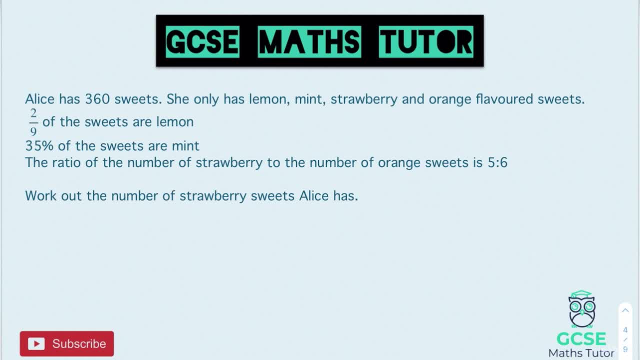 go and we'll go over the answers in a sec. Okay then. so let's have a look. Let's have a look at this. So, for the fraction of the amount you've got to work out, 2 ninths that are lemon. So if we get 2 ninths of 360, we know that 1 ninth is going to equal 80,. 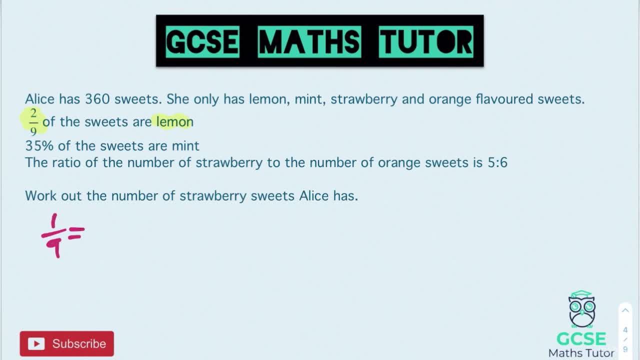 that's why 2 ninths is going to equal 80, but 1 ninth is going to equal 40, and then 2 ninths is going to equal 80. But again showing you're working out how you, divided by 9 to get 40, and then labelling the information. so we've got that for in a moment. 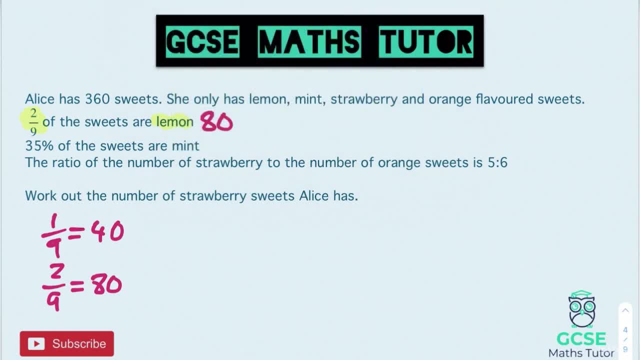 Onto the next part. you've got the 35%, and let's just highlight this: 35% are mint- and to work out that you're going to get that your 10% is 36,, you're going to get that your 5% is 18, and then build that up so that you have 3 of the 36's and 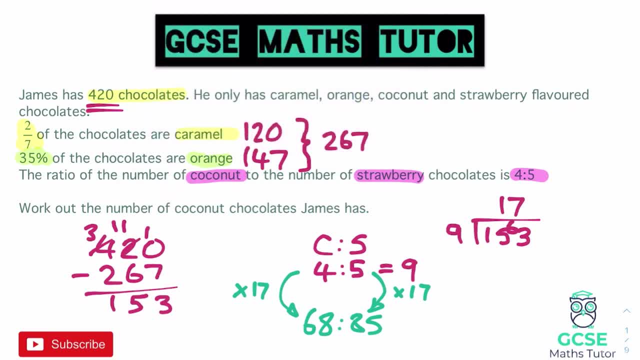 That is all of our amounts there. If we apply that back to the question, underneath coconut there we've got 68. And underneath strawberry we have 85. Now the question here did only say: work out the number of coconut chocolates that James. 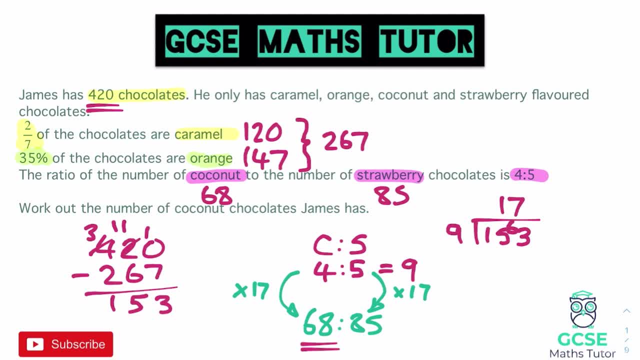 has. So for our final answer we would say 68,, as that was the amount of coconut that we had. So we worked out that ratio. So there we go. There was a lot going on in that question. You had to work out a fraction of an amount, a percentage of an amount, finding out what. 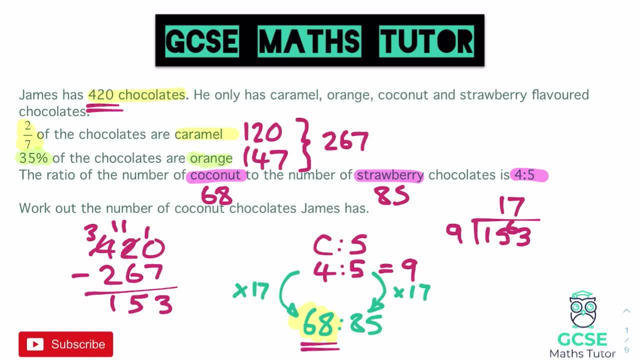 was left and then sharing that in a ratio. So a lot going on in this question, but I'm going to give you a question very, very similar to this so you can have a go, have a practice with some of these methods. 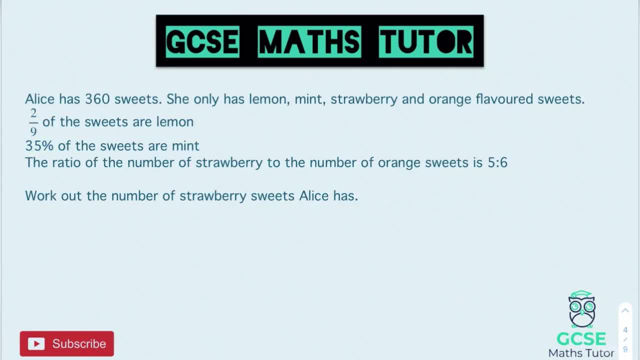 So let's have a look at that now. Okay, so a very similar question for you to practice. So pause the video there, have a go and we'll go over the answers in a sec. Okay then. so let's have a look at this. 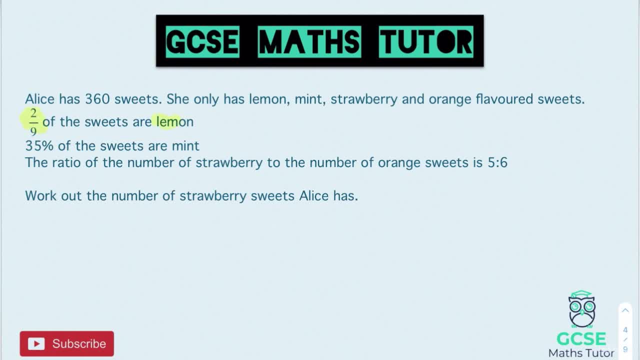 So for the fraction of the amount, you've got to work out two-ninths that are lemon. So if we get two-ninths of 360, we know that one-ninth is going to equal 80.. That's well, two-ninths is going to equal 80, but one-ninth is going to equal 40, and 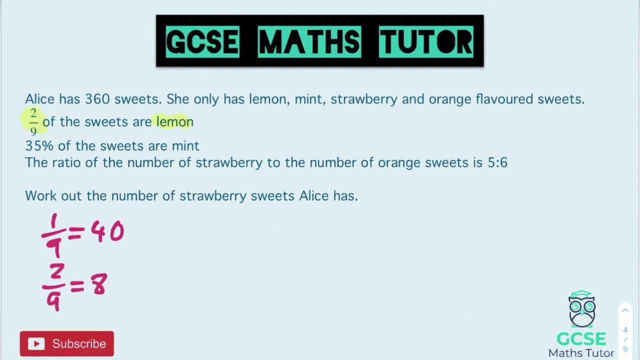 then two-ninths is going to equal 80. But again, showing you're working out how you divided by nine to get 40, and then labeling the information. So we've got that for in a moment Onto the next part. you've got the 35% and let's just highlight this. 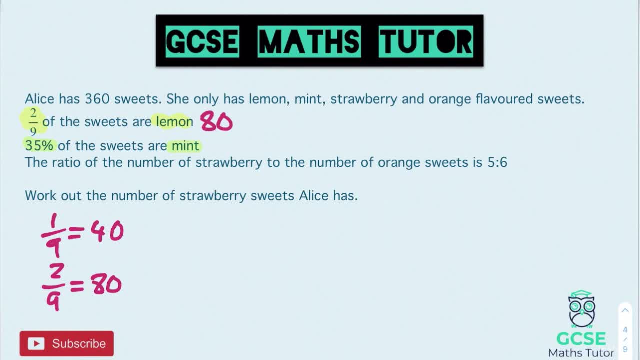 35%- Our mint- and to work out that you're going to get your 10% is 36,. you're going to get that your 5% is 18, and then build that up so that you have three of the 36s and one. 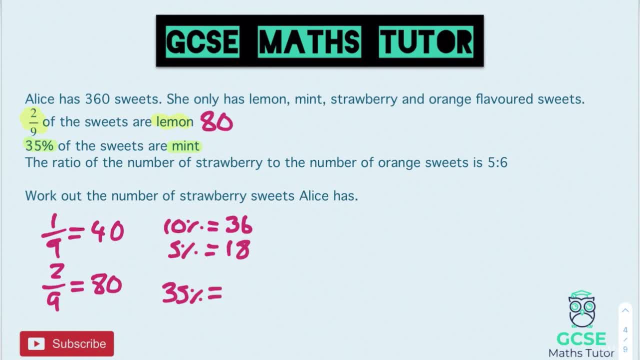 of the 5%, which is the 18, and 35%, in total equals 126.. So we have 126 in total. that's a mint Again. now you can add those both together and that gives you 206 in total and you're. 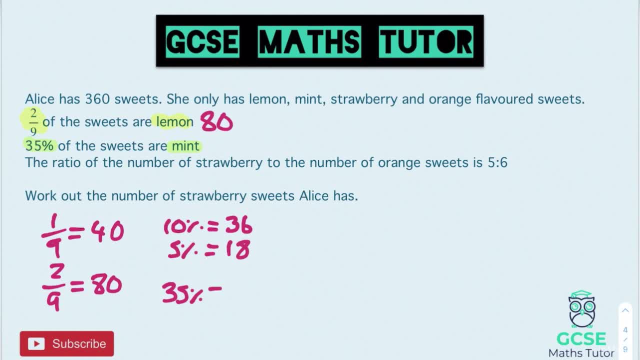 1 of the 5%, which is the 18, and 35%, in total equals 126. So we have 126 in total. that's a mint Again. now you can add those both together and that gives you 206 in total. 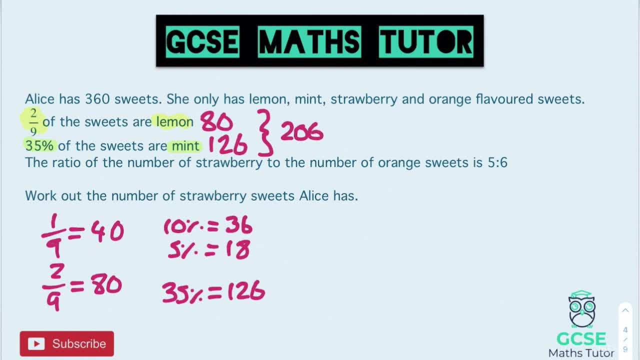 And you're going to have to take that away from the total 360 in order to get our amount that can be shared in the ratio. So if we do 360, and we take away 206, you should have got the answer there 254.. Sorry, that's wrong- 154.. There we go, 154. 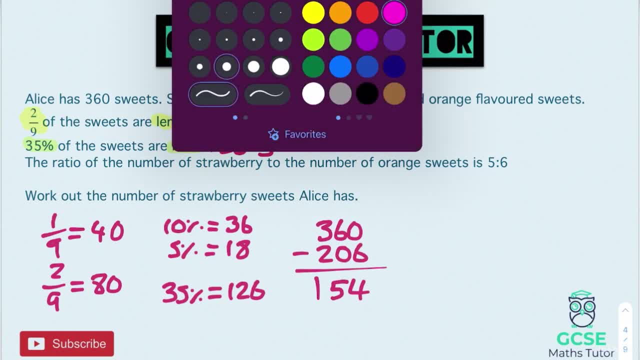 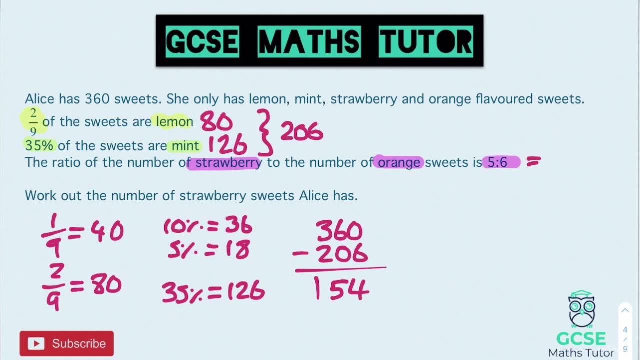 Now onto the next part. you're going to share that in the ratio. So if we have a look, the information that we're given is that strawberry and orange are mint. Orange is in the ratio 5 to 4, so that in total is 11 parts. So you have to divide 154. 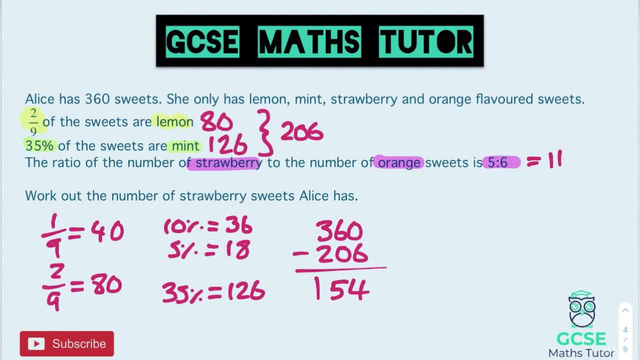 by 11, and that gives you a total. and if we write that down here, divide by 11, that gives you a total per part of what is that? 14.. There we go, so we get 14 in total. 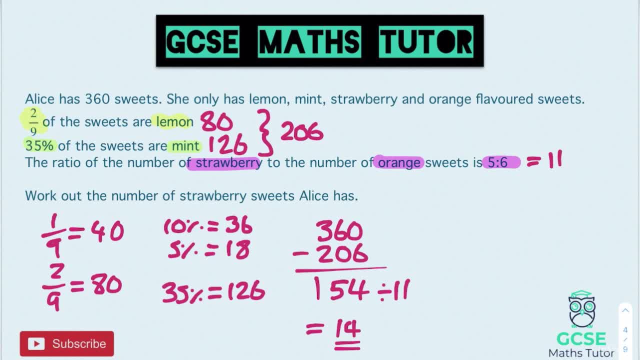 Now we have our last step here, which is to multiply the ratio. so we have strawberry and orange, Which is again 5 to 6, and we want to multiply both of those by 14, which gives us 70 for strawberry. that's not 70, so 70 for strawberry and for the 6, we'll times that by 14, and 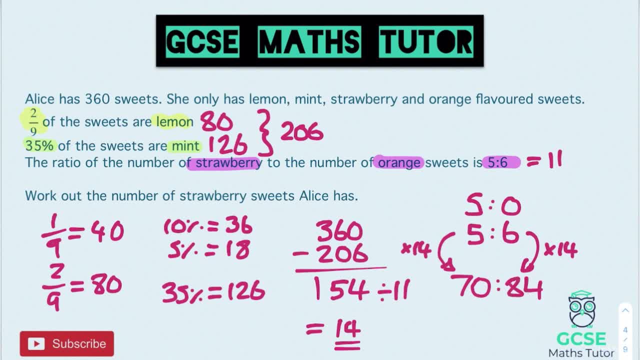 that is 84. At this point here, add those two together, just to double check: 70 and 84,. add together to make the 154.. So we should have a correct answer there. So, looking back at the question, what did it ask for? it said the number of strawberry. 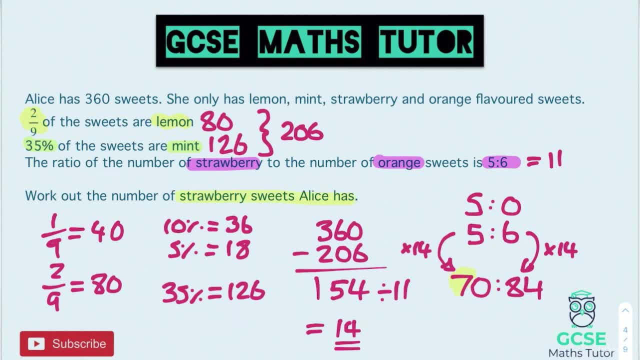 sweets that Alice has strawberry was the 5 parts, which was the 70, so our final answer for that question was 70.. There we go, right. let's have a look at one more type of question. Okay, so this question here. then we've got a lot of information. it says: on Saturday: 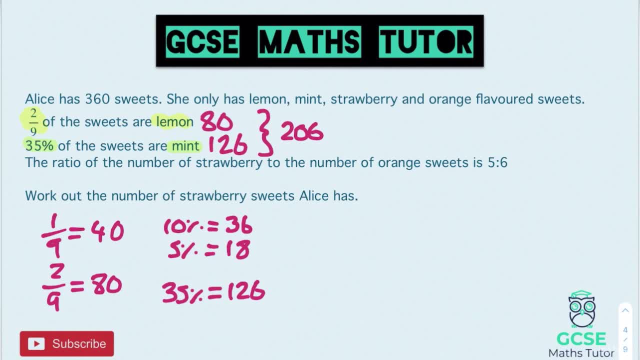 going to take that away from the total 360 in order to get our amount that can be shared in the ratio. So if we do 360, and we take away 206,, you should have got the answer there 254.. Sorry, that's wrong: 154,. there we go, 154. 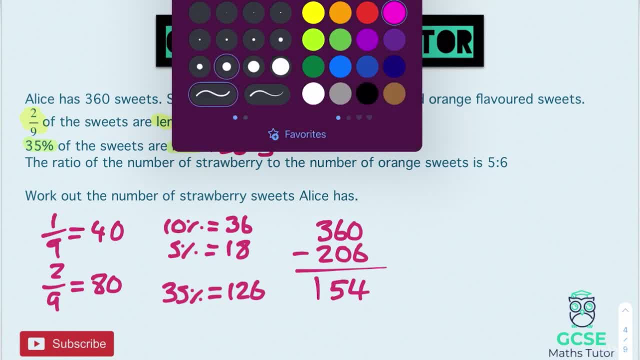 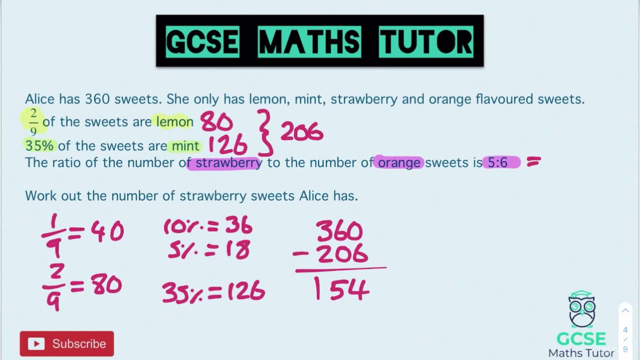 Now onto the next part. you're going to share that in the ratio. So if we have a look, the information that we're given is that strawberry and orange is in the ratio Five to four, so that in total is 11 parts. 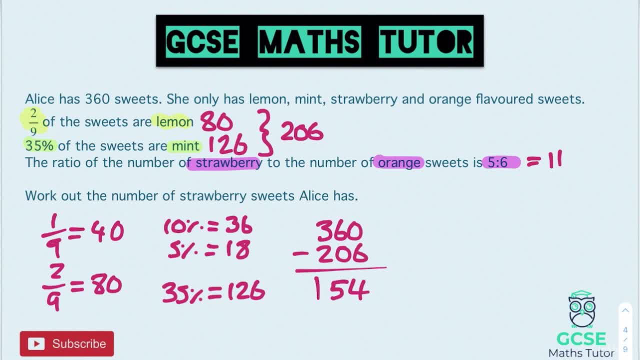 So you have to divide 154 by 11, and that gives you a total. and if we write that down here, divide by 11, that gives you a total per part of what is that? 14,. there we go. 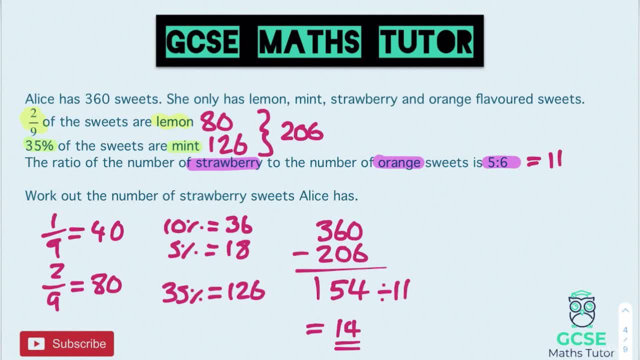 So we get 14 in total. Now we have our last step here, which is to multiply the ratio. so we have strawberry and orange, which is again five to six, And we want to multiply both of those by 14, which gives us 70 for strawberry. that's. 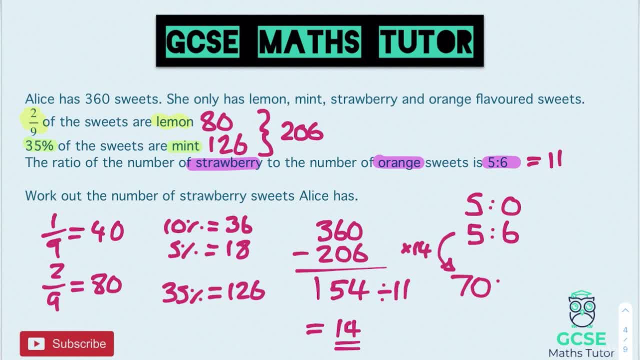 not 70,. so 70 for strawberry and for the six. we'll times that by 14, and that is 84. At this point here, add those two together, just to double check: 70 and 84, add together. 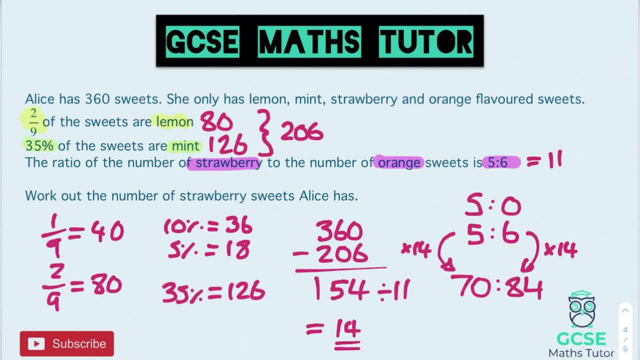 to make the 154. So we should have a correct answer. So, looking back at the question, what did it ask for? it said the number of strawberry sweets that Alice has strawberry was the five parts, which was the 70, so our final. 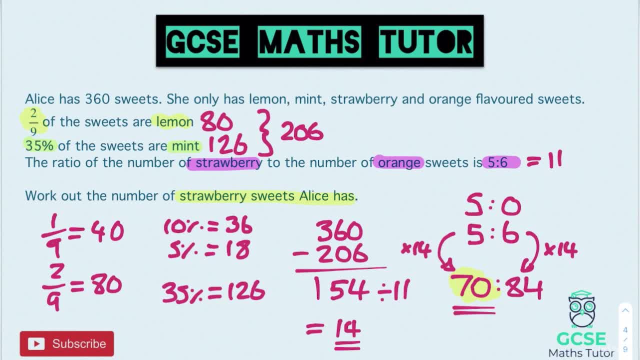 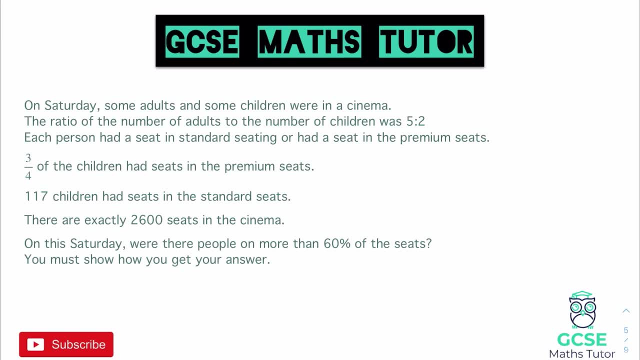 answer for that question was 70.. There we go. right, let's have a look at one more type of question. Okay, so this question here, then we've got a lot of information. it says: on Saturday, some adults and some children were in a cinema. 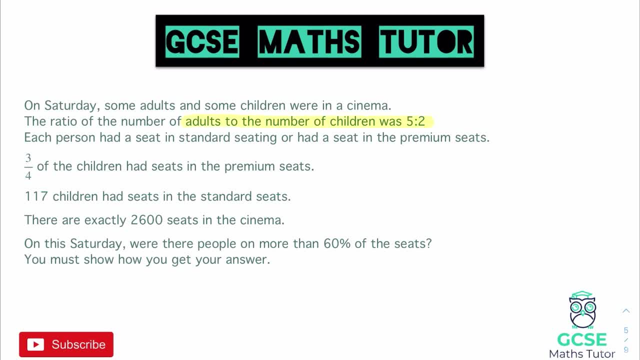 It says, the ratio of the number of adults to the number of children was five to two, and each person had a seat in standard seating or had a seat in the premium seats. Three quarters of the children had a seat in the premium seats and 117 children had 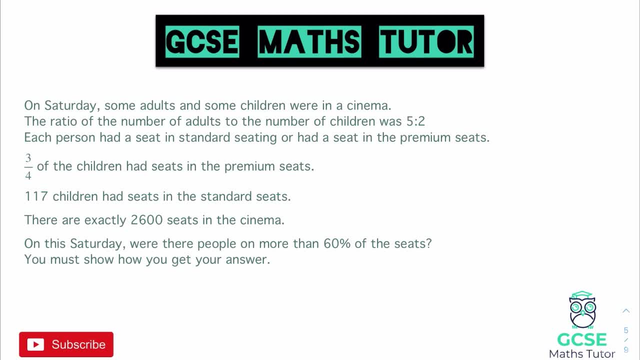 some adults and some children were in a cinema. It says the ratio of the number of adults to the number of children was 5 to 2. And each person had a seat in standard seating or had a seat in the premium seats. Three quarters of the children had a seat in the premium seats and 117 children had 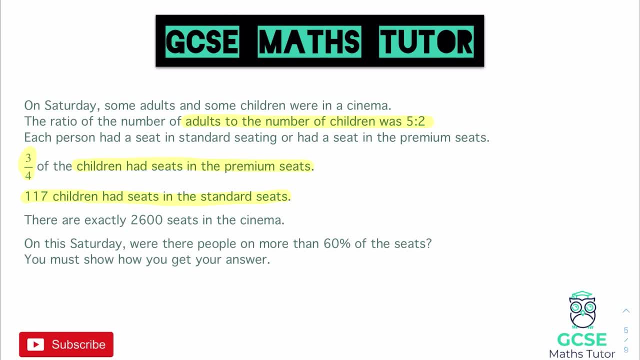 a seat in the standard seats And there are exactly 2,600 seats in the cinema. Let's just highlight that in a different colour And it says on the Saturday were there people on more than 60% of the seats. So there's a couple of different ways that you could approach this. 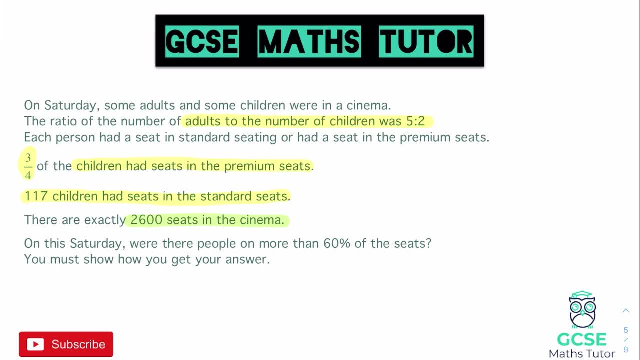 What we could do is we could straight away work out that 60%, which seems a little bit counterintuitive as it's the last line in the question. But if we work out that 60% straight away, we'll know what kind of number we're aiming for here. 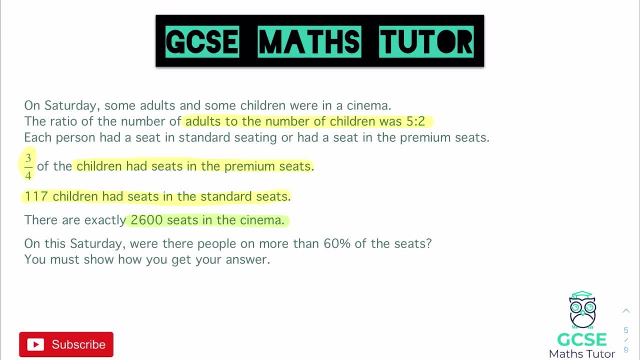 So we could work out that 60% And again, depending on whether you are using a calculator or not, will depend on how you approach that. But if we do that without a calculator, because that's relatively simple for us to do- we can just work out this 60% to start with. 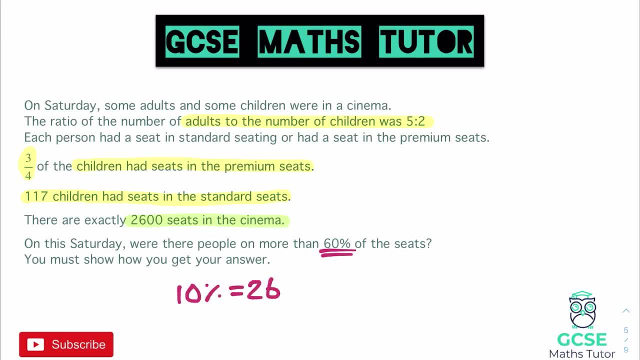 So 10% would equal 260.. And then we times that by six to get our 60%. And if we just do that using column multiplication, just to get our answer nice and quick, six times zero is zero, six times six is 36,. 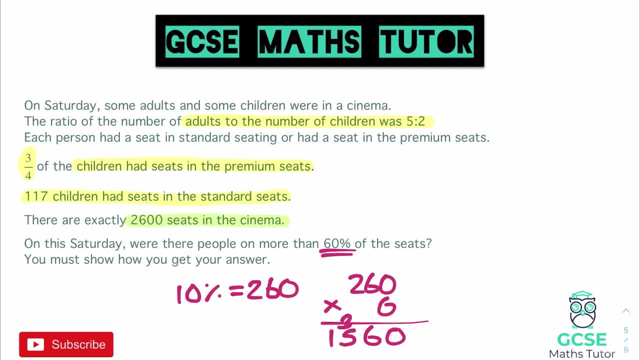 and six times two is 12.. So that's 1,560.. Now, on a question like this, you never know in an exam that may have just got you a mark. So well worth working that out if that's the nice easy step to go for this question. 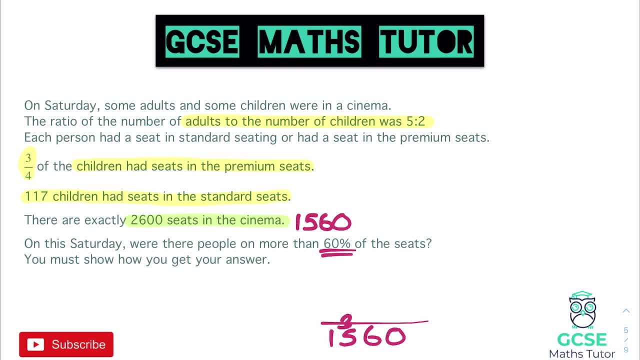 So let's get rid of that And obviously always leave your working out again, but we'll get rid of that And we'll just have a look at going back to the start. So it says adults to children was five to two, And then it gives us some information. 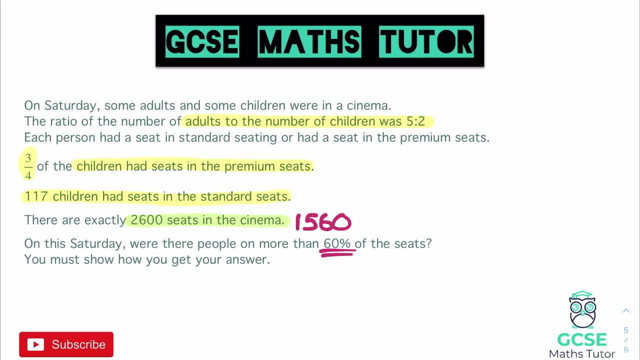 about where they sat. We know that three quarters of them had seats in the premium seats and 117 children were in the standard seats. Now, both of those bits of information are just about the children. So if three quarters of them were in the premium seats, 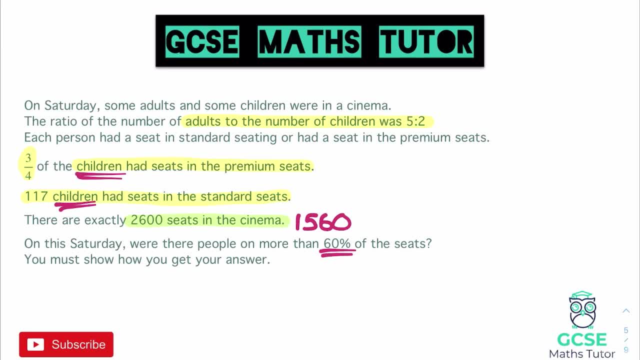 the other quarter must have been in the standard seats And it tells us that that was 117 children. So we'll know that that was 117 children. So we'll know if this one is three quarters and this one was one quarter because it's the rest of the children. 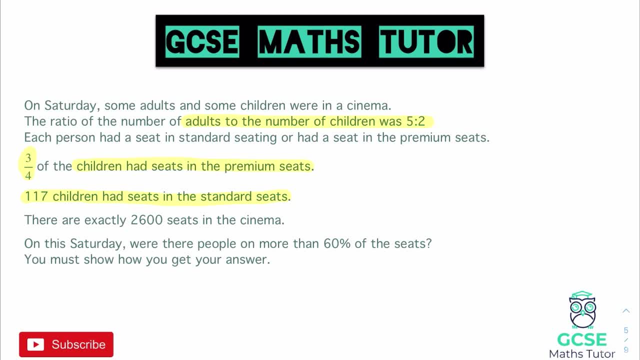 a seat in the standard seats And there are exactly 2,600 seats in the cinema. let's just highlight that in a different colour And it says on the Saturday were there people on more than 60% of the seats. So there's a couple of different ways that you could approach this. 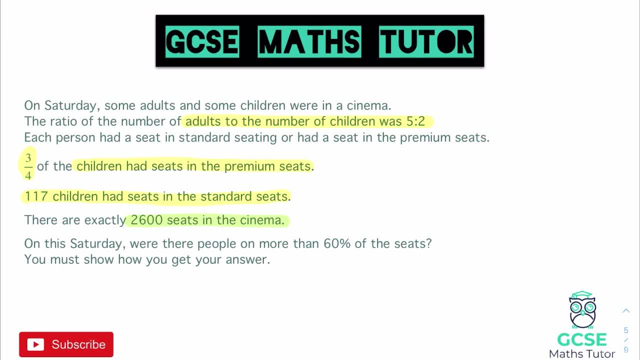 What we could do is we could straight away work out that 60%, which seems a little bit counter-intuitive as it's the last line in the question. but if we work out that 60% straight away, we'll know what kind of number we're aiming for here. 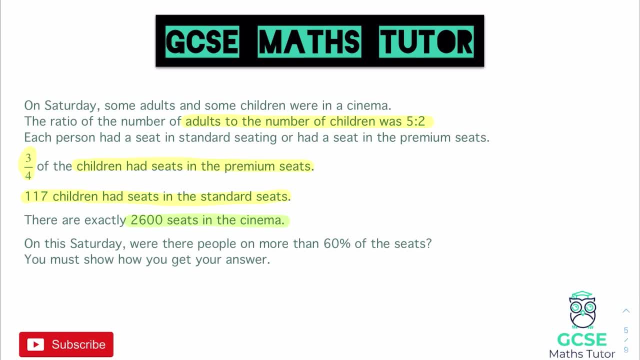 So we could work out that 60% and again, depending on whether you are using a calculator or not, will depend on how you approach that. but if we do that without a calculator, because that's relatively simple for us to do- we can just work out this 60% to start with. 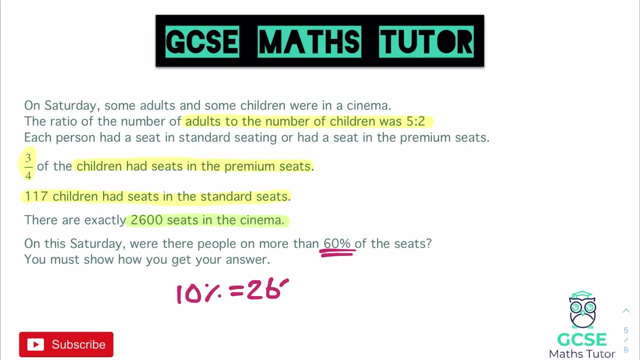 So 10% would equal 260.. And then we'd do that, So 10% would equal 260.. And then we'd do that, So 10% would equal 260.. And if we just do that using column multiplication, just to get our answer nice and quick- 6 times. 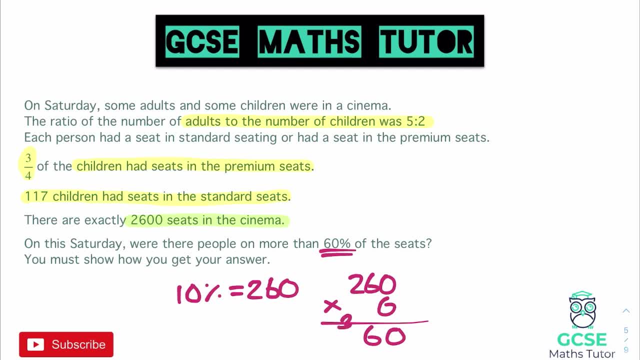 0 is 0,, 6 times 6 is 36, and 6 times 2 is 12,, so that's 1,560.. Now, on a question like this, you never know, in an exam, that may have just got you a mark. 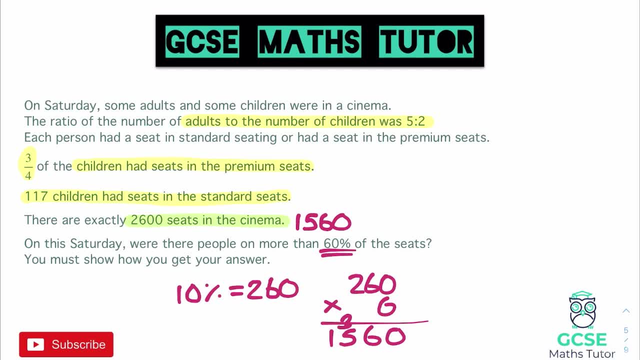 So well worth working that out if that's the nice easy step to go for this question. So let's get rid of that and obviously always leave your working out again. but we'll get get rid of that and we'll just have a look at going back to the start. So it says adults to 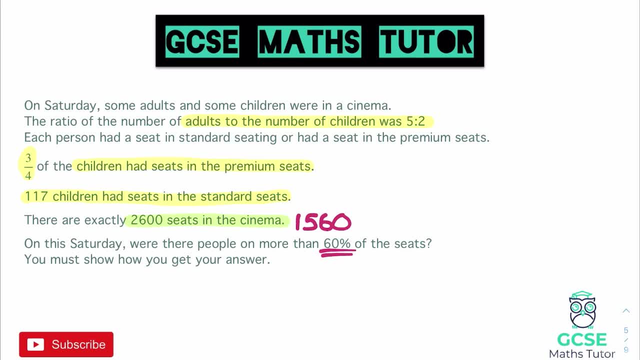 children was five to two, and then it gives us some information about where they sat. We know that three quarters of them had seats in the premium seats and 117 children were in the standard seats. Now, both of those bits of information are just about the children. so if three quarters of 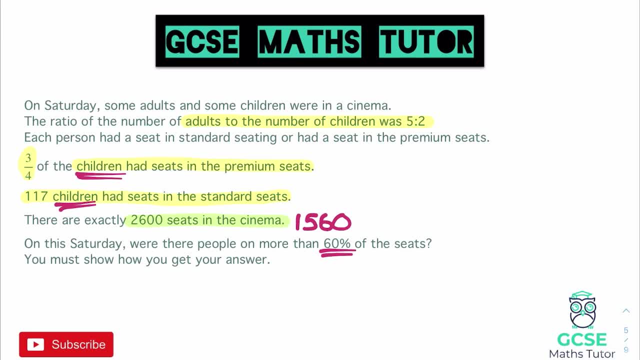 them were in the premium seats. the other quarter must have been in the standard seats and it tells us that that was 117 children. So we'll know if this one is three quarters and this one was one quarter, because it's the rest of the children and it tells us that that one quarter is equal to 117. 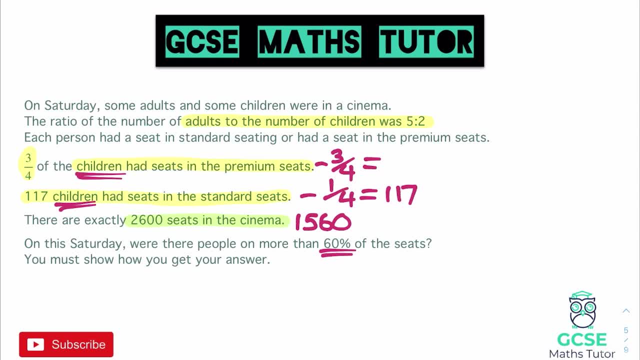 we just want to know what the three quarters is equal to, and we know if one quarter is 117. in order to get three quarters, we just have to multiply that by three. So if we multiply that by three, that is going to tell us the amount of children that were in the premium seats. 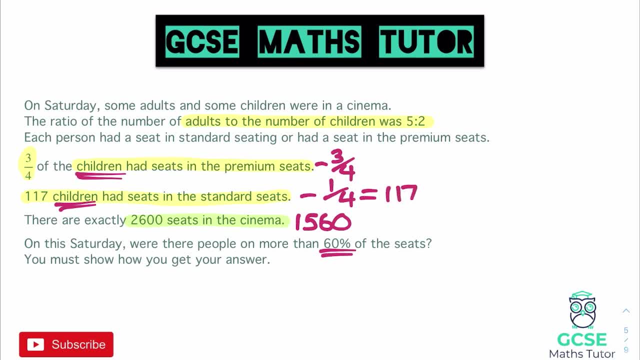 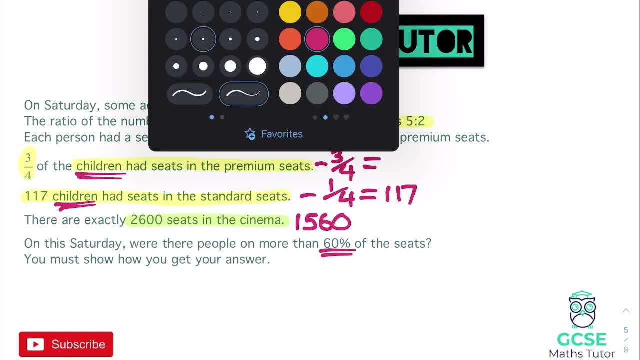 And it tells us that that one quarter is equal to 117.. We just want to know what the three quarters is equal to, And we know if one quarter is 117, in order to get three quarters, we just have to multiply that by three. 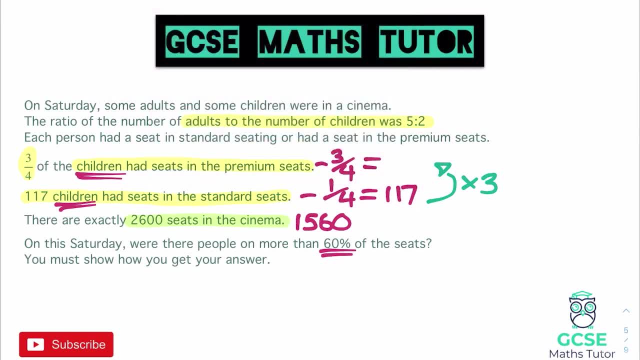 So if we multiply that by three, that is going to tell us the amount of children that were in the premium seats. So 117 times three. And again you've just got to do some working out. Again you can either multiply it by three. 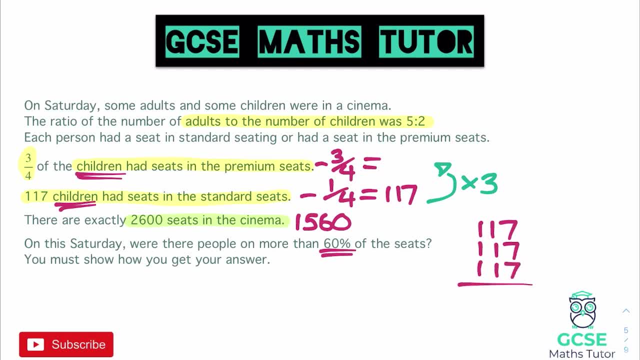 or you could just add that together three times. whichever you prefer, I'm going to use a combination of methods here. So that adds up to 21.. That adds up to five, And that adds up to three, So that is 351.. 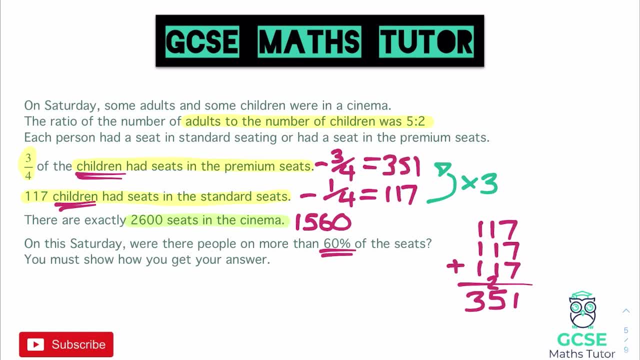 So we know that there are 351 children that are in the premium seats. Let's get rid of that working out, because we now have quite a lot of information. We know that the first thing we worked out was trying to see if they filled 1,560 seats. 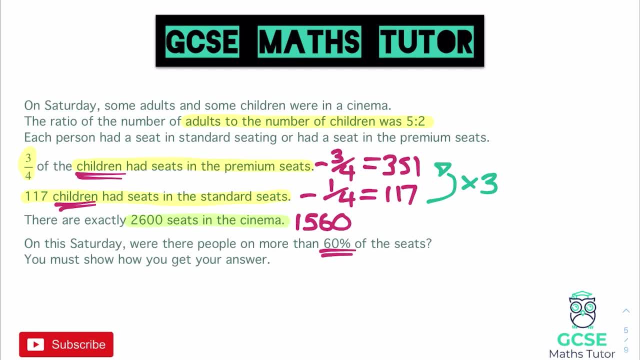 And now, in this second bit of information, we've actually worked out the total number of children. We have 351 that are in the premium seats and 117 that are in the standard seats. So if we add those both together, we have eight, six and four. 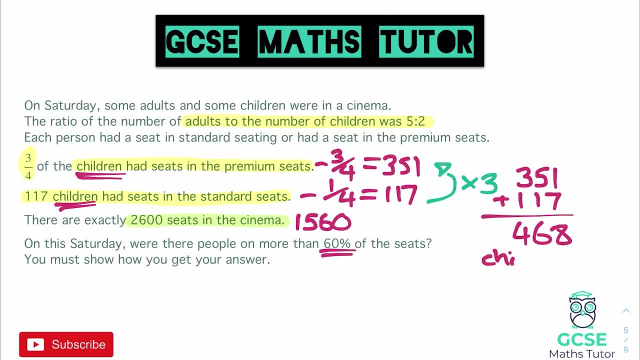 So 468 children. Now we obviously just want to work out how many adults there are. So we know that there are 468 children, but how are we going to get to the adults? So it tells us the ratio of adults to children at the start. 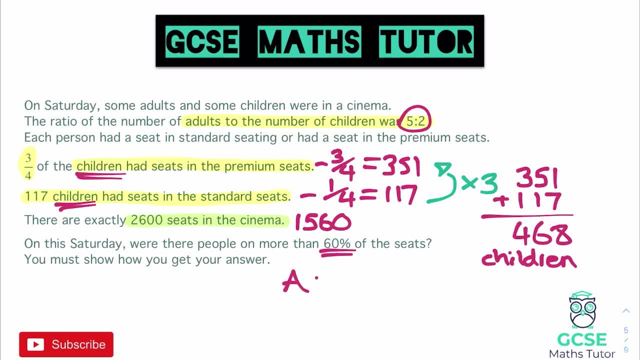 Just over here And it tells us that the ratio of adults to children is five to two And we've already worked out that the children in that ratio is 468.. So we're using a different part of our ratio here. We're not just sharing in a ratio. 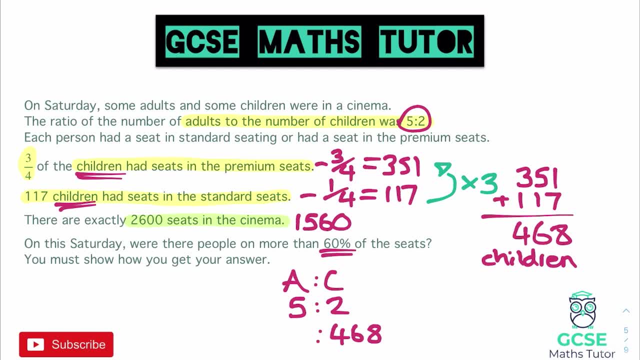 We're actually working backwards because we've already been given one of the numbers. So, in order to get back to one part, we could divide that by two, And that would allow us to then figure out the other way around, what we would have to have multiplied by essentially. 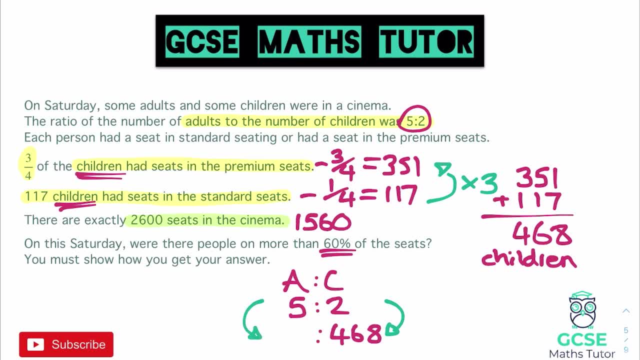 to get our number down. So let's go down here to figure out the amount of adults. So if I want to work that out to the side, I can do 468 divided by two, which tells me what one part would be worth. 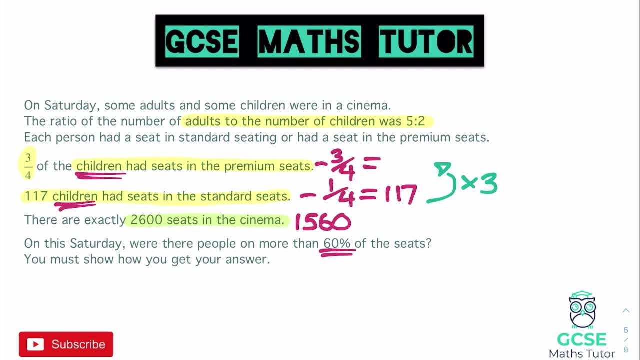 So 117 children were all in the premium seats. So we'll know what the three quarters was and times three and again. you've just got to do some working out again. you can either multiply it by three or you could just add that together three times. whichever you prefer, I'm going to use a 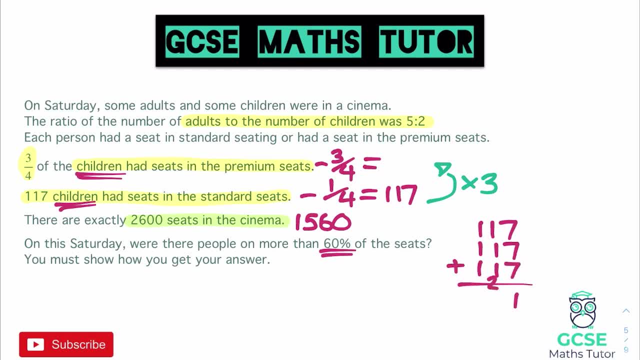 combination of methods here. so that adds up to 21, that adds up to five and that adds up to three. so that is 351. so we know that there are 351 children that are in the premium seats. let's get rid of that working out, because we now have quite a lot of information. we know that the first 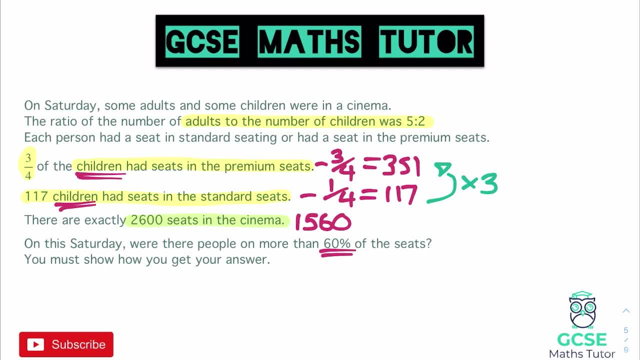 thing we worked out was to try to see if they filled 1560 seats, and now, in this second bit of information, we've actually worked out the total number of children we have: 351 that are in the premium seats and 117 that are in the standard seats. so if we add those both together, we have 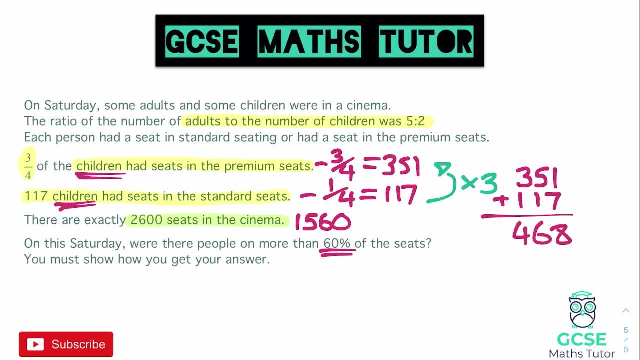 eight, six and four, so 468 children. now we obviously just want to work out how many adults there are. so we know there are 400 and 168 children, but how are we going to get to the adults? so it tells us the ratio of adults to. 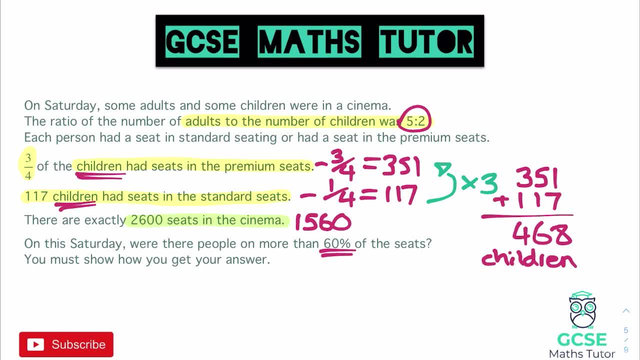 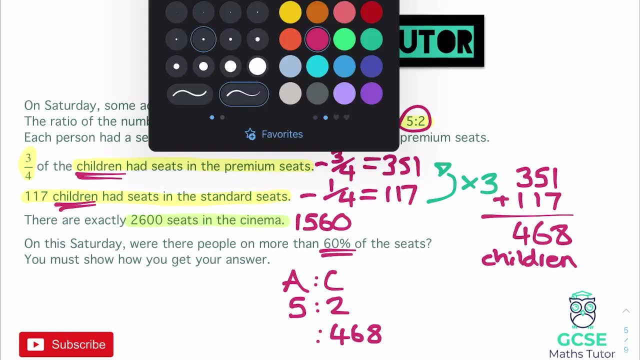 children at the start just over here, and it tells us that the ratio of adults to children is five to two and we've already worked out that the children in that ratio is 468. so we're using a different part of our ratio here. we're not just sharing in a ratio, we're actually working backwards. 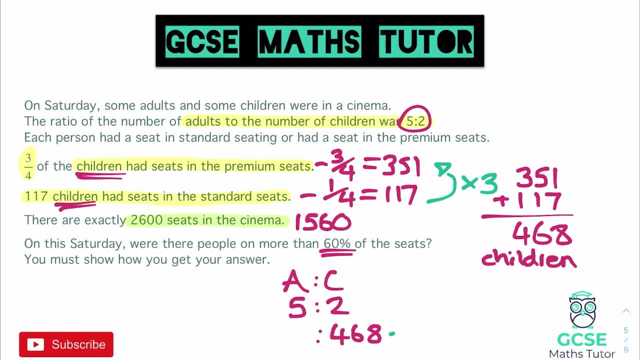 because we've already been given one of the numbers. so, in order to get back to one part, we could divide that by two, and that would allow us to then figure out the other way around: what we would have to have multiplied by essentially to get our number down here, to figure out the amount of adults. 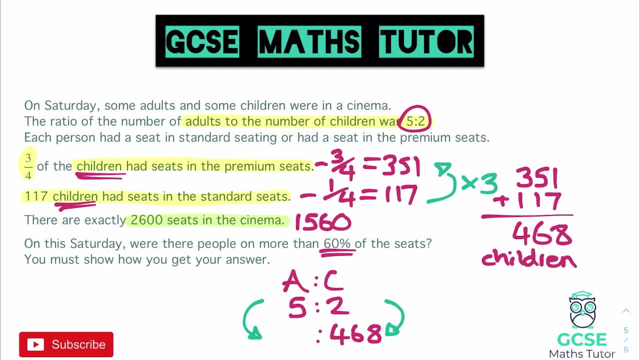 so if i want to work that out to the side, i can do 468 divided by two, which tells me what one part would be worth, and that answer comes out as 234. so we must have multiplied by 234 per part in order to share that ratio out. so times 234. so that means we've got the number of adults that are in the 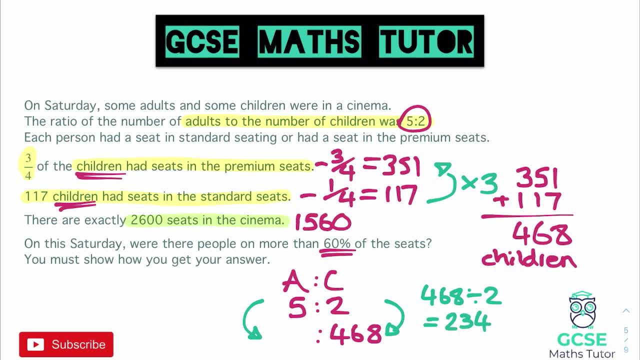 And that answer comes out as 234.. So we must have multiplied by 234 per part in order to share that ratio out. So times 234.. So that means, in order to get the total amount of adults, we're going to have to times by 234. 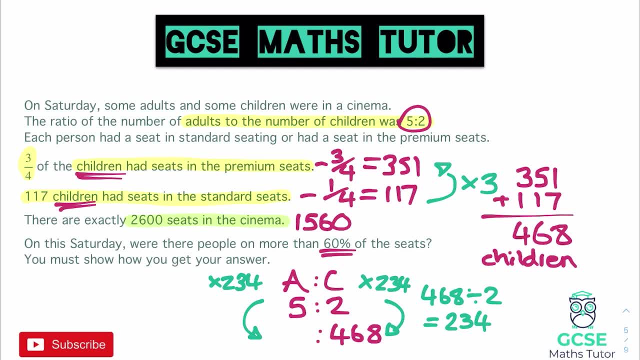 Again, if this is non-calculator, you're going to have to do some working out there. Or you could just apply a little bit of a trick for timesing by five, which is to times by 10 and half it, Although you might argue it's probably just quicker. 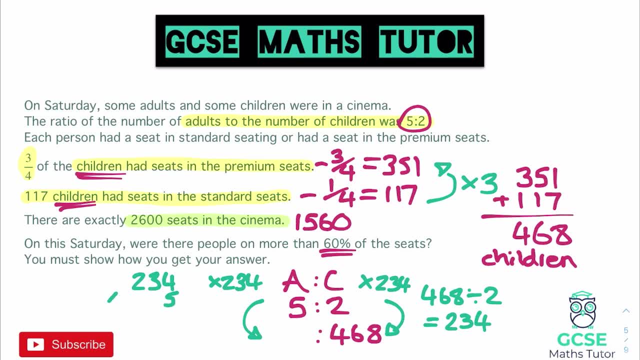 to do 234 times five to the side and just get that correct. So five times four is 20.. Three times five is 15.. Add the two is 17.. And then two times five is 10, plus the one is 11.. 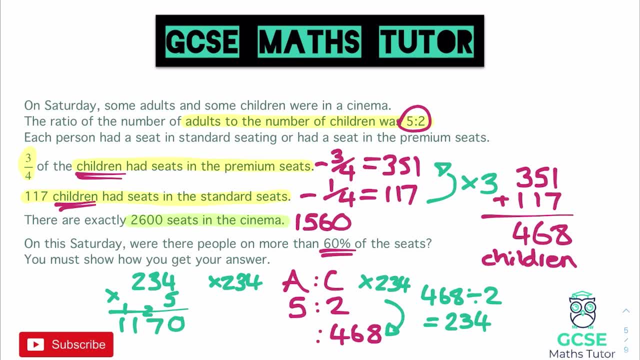 So, in terms of working this out- and we're going to need a bit more space there- Let's get rid of that arrow. We've got 1,100.. We've got 1,170 adults And to get there, we times by 234.. 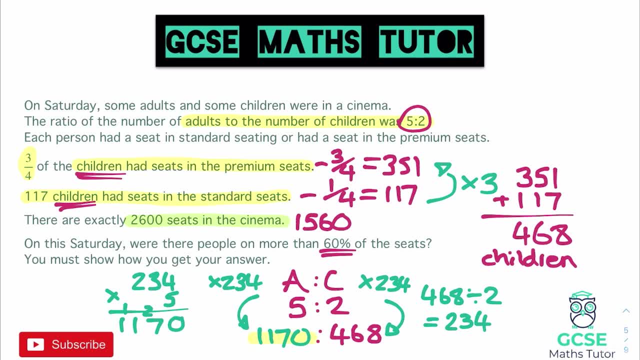 Okay, so we've got quite a bit of information now. We've got 1,170 adults And we've got 468 children, And it said is 60% of the seats filled, And we already worked out that in order to fill that. 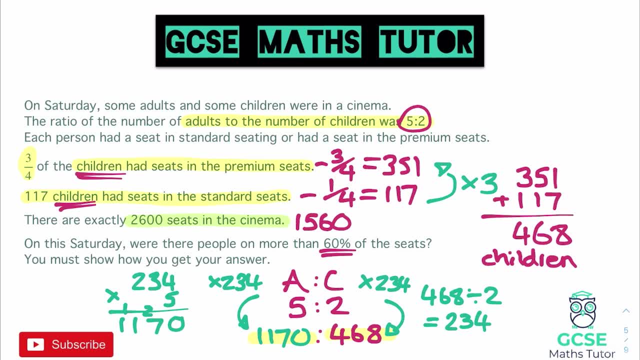 we needed to fill 1,560 seats. So now we have all this information And let's get all of this out of the way- We can actually finish this question off, because we can actually just add these two together And that's going to give us the total amount of people at the cinema. 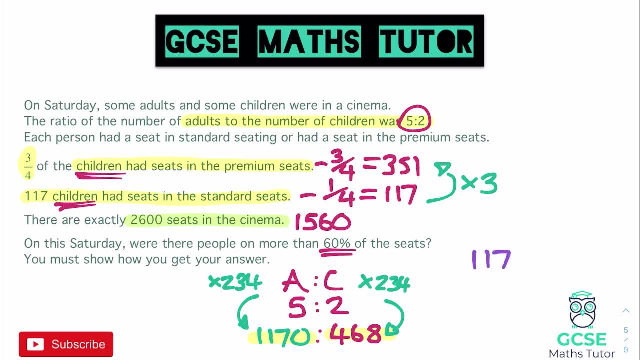 So, to finish this off, we do 1,170, the total amount of adults, Add 468, the total amount of children. That adds up to 5,6,1,, 1,638,, which is greater than 1,560.. 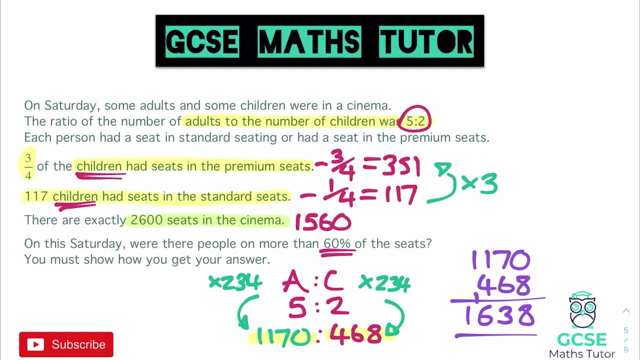 So where it says, were there people on more than 60% of the seats, We would say yes, And you could either then write a sentence to say 1,638 is more than 1,560. Or you could just say it as an inequality. 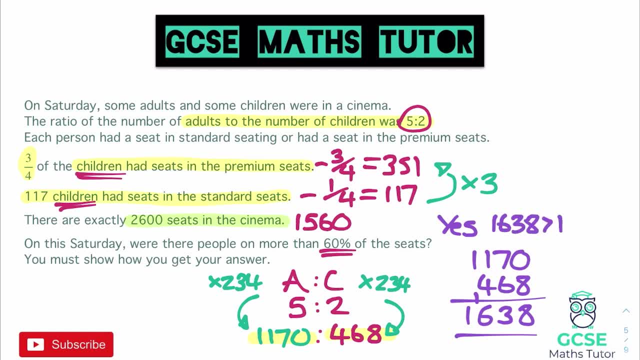 1,638 is greater than 1,560.. And there we go. And don't forget to write your conclusion here, as it does say that. And don't forget the question does say you must show how you get your answer. So all of that working out is essential. 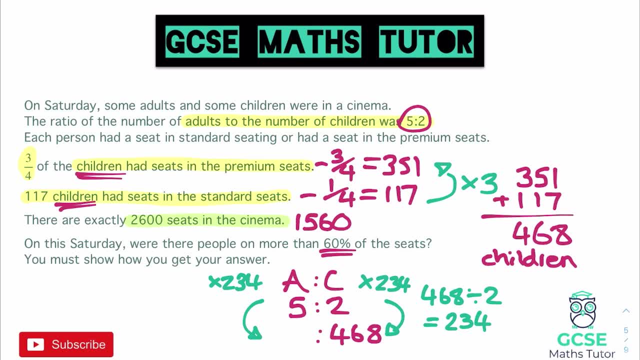 total number. to get the total amount of adults, we're going to have to times by 234. again, if this is non-calculator, you're going to have to do some working out there, or you could just apply a little bit of a trick for timesing by five, which is to times by 10 and half it, although you might argue. 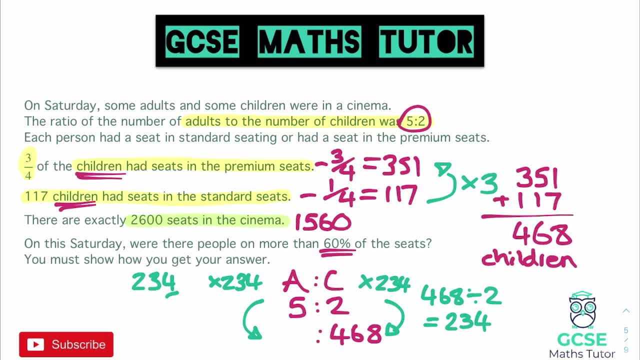 it's probably just quicker to do 234 times 5 to the side and just get that correct. so 5 times 4 is 20, 3 times 5 is 15, add the 2 is 17 and then 2 times 5 is 10 plus the 1 is 11. 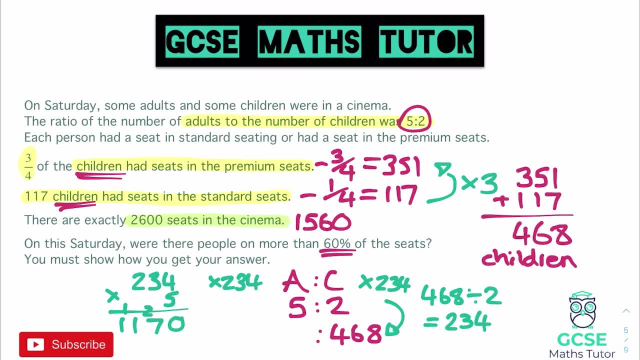 in terms of working this out and we're going to need a bit more space there. let's get rid of that arrow. we've got 1170 adults and to get there, we times by 234.. Okay, so we've got quite a bit of information now. we've got 1170 adults and we've got 468 children and it said is 60% of the seats. 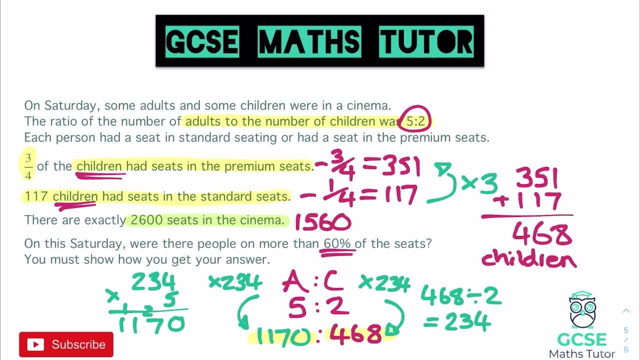 filled, and we already worked out that in order to fill that, we needed to fill 1560 seats. So now we have all this information and let's get all of this out the way, we can actually finish this question off, because we can actually just add these two together and that's going to give us 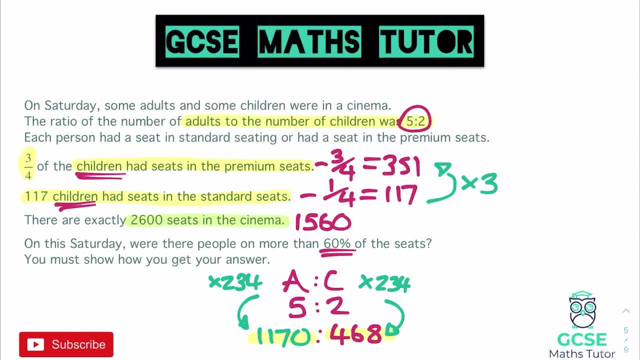 the total amount of people at the cinema. So to finish this off, we do 1170, the total amount of adults, add 468 the total amount of children. that adds up to 5, 6, 1, 1638, which is greater than 1560.. 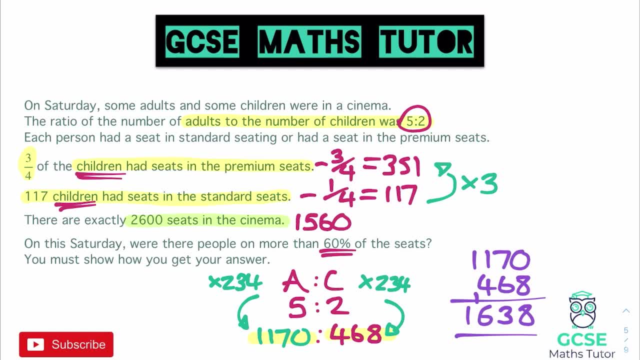 So where it says it was where there more, where there people are more than 60% of the seats, we would say yes, and you could either then write a sentence to say 1638 is more than 1560, or you could just say, as an inequality, 1638 is greater than 1560. and there we go, and don't forget to write your conclusion. 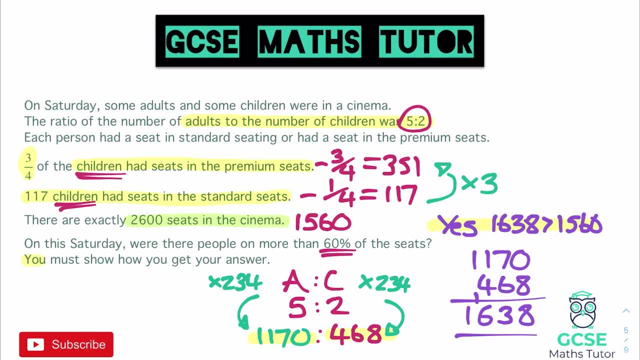 here, as it does say that and, don't forget, the question does say you must show how you get your answers. that's working out as essential. There's a lot of information in that question. we've gone through quite a lot there. we're reversing the kind of fractions, reversing the ratio. 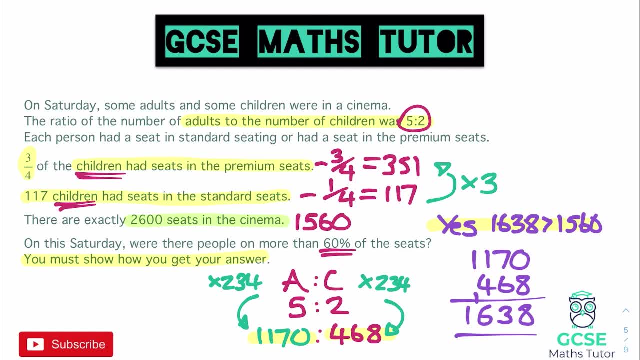 Now, there's a lot of information in that question. We've gone through quite a lot there. We're reversing the kind of fractions, reversing the kind of numbers. So we're reversing the kind of fractions, reversing the kind of numbers. But I do have a question for this, for you to practice. 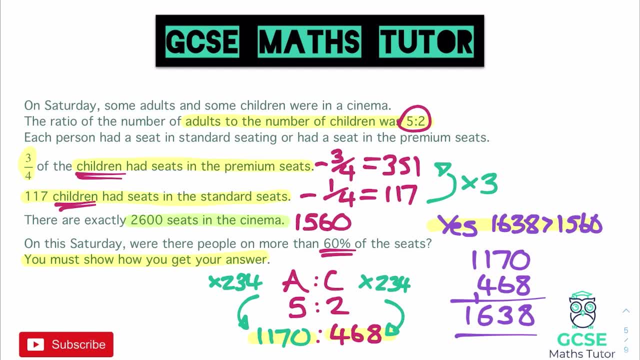 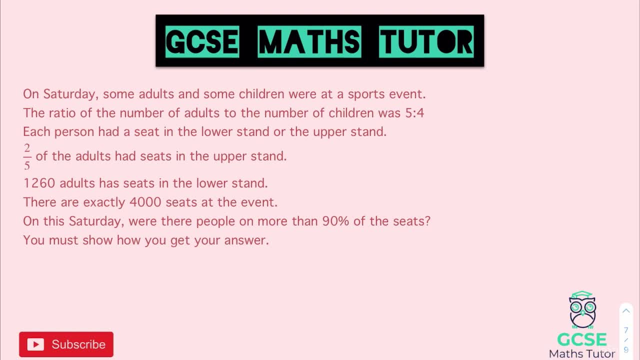 So if you need to go back, listen to that again, Or if not and you think you can have a go, let's have a look at a question for you. Okay, so here is your last question, Very similar to the one we just had a go at. 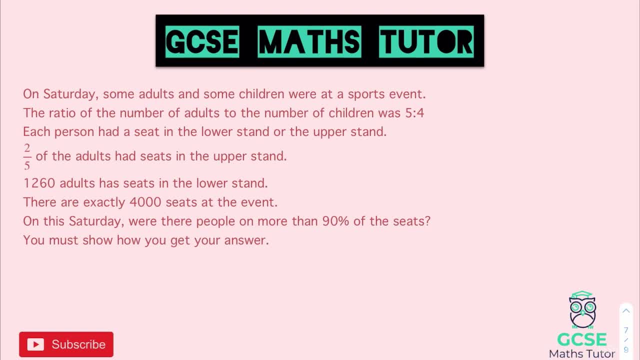 So read this carefully, highlight any of the key information and pause the video and we'll go over the answer in a sec. Okay, so let's have a look. I've got some quite large numbers in this question, But it says that the ratio of adults to children at a sports event was 5.2. 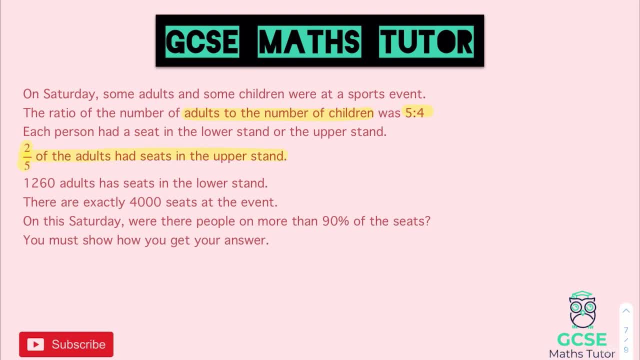 It says that two-fifths of the adults were in the upper stand, 1,260 adults were in the lower stand and there were 4,000 seats at the event, And it says were there more than 90% of those filled. 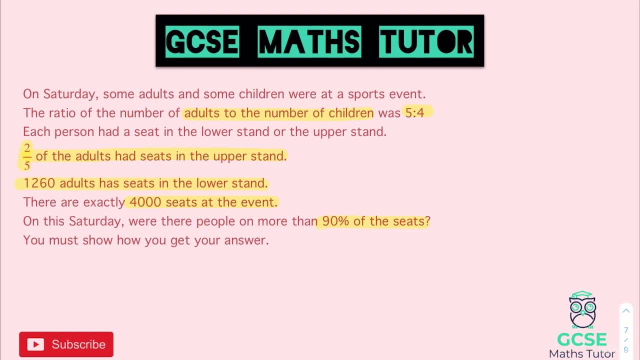 So again, the first thing that I would work out here is 90% of 4,000. And if you work out 10%, it comes out as 400. And you can actually just take that away from the 4,000,. 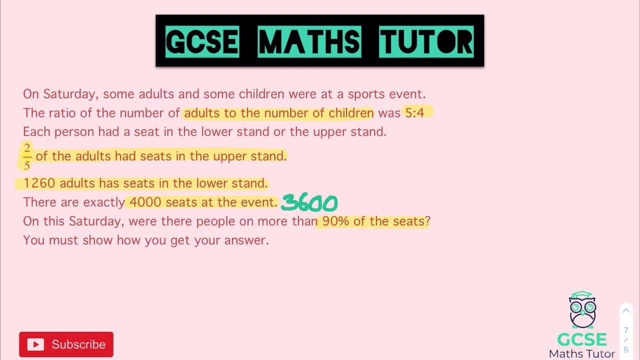 which gives you 3,600 seats that we're looking to see if they're filled. Or you could just do the 4,000, and times it by 9,, which again gives you the 3,600.. Moving on then. 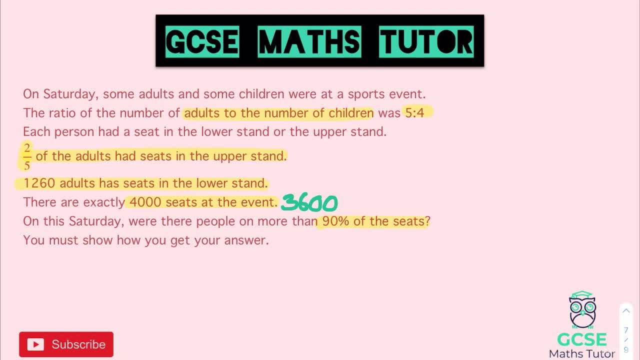 Now it says that two-fifths of the adults had seats in the upper stand. So if that is two-fifths, then the amount of adults in the lower stand must have been three-fifths, And we know that that three-fifths is equal to 1,260.. 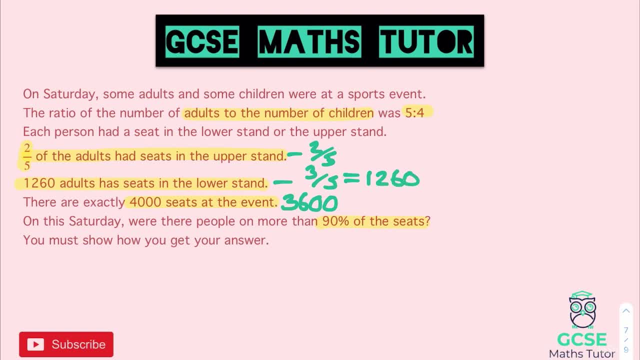 Now, this is actually the one step in here which is a little bit harder than the last one, Because to get three-fifths to two-fifths, that's a little bit more complicated And in order to get that down, 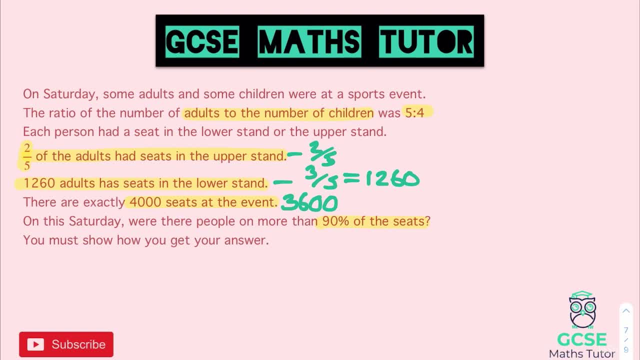 so one-fifth. you would have to divide that by three, as that is currently three-fifths, And if we divide that by three, that would give us that one-fifth is going to be equal to 420.. And again, just writing the working out down there: 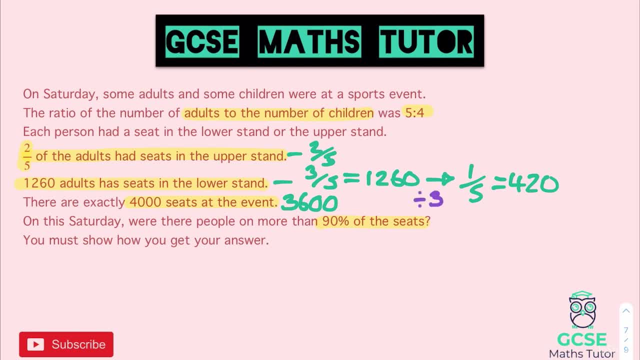 we divided that by three, Remember, three-fifths divided by three would give us one-fifth. We can then multiply that by two and that would give us the amount for two-fifths. And if we multiply 420 by two, you get 840.. 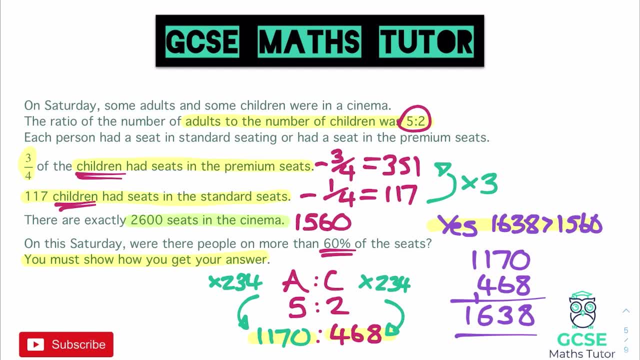 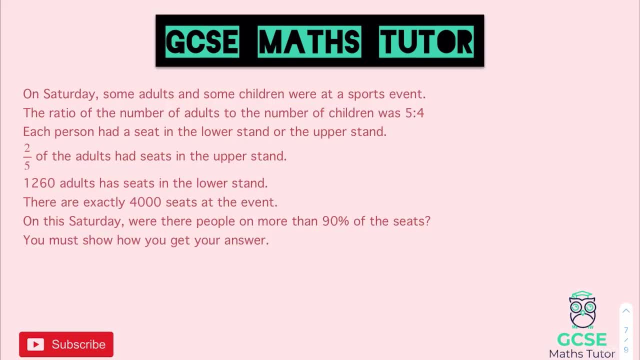 but I do have a question for this, for you, to practice. so if you need to go back, listen to that again, or if not anything, you can have a go, let's have a look at a question for you. Okay, so here is your last question, very similar to the one we just had a go out to read carefully. 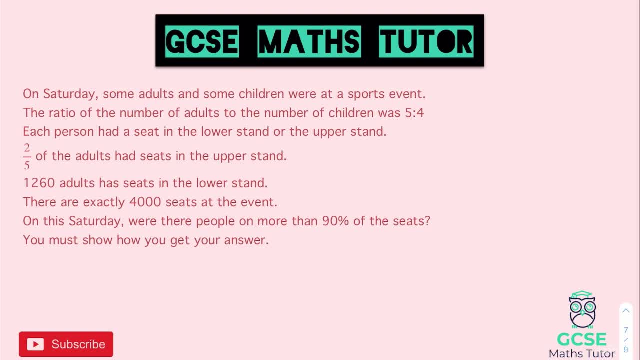 highlights any of the key information and pause the video and we'll go over the answer in a while, okay, Okay, so let's have a look. I've got some quite large numbers in this question, but it says that the ratio of adults to children at a sports event was 5 to 4.. 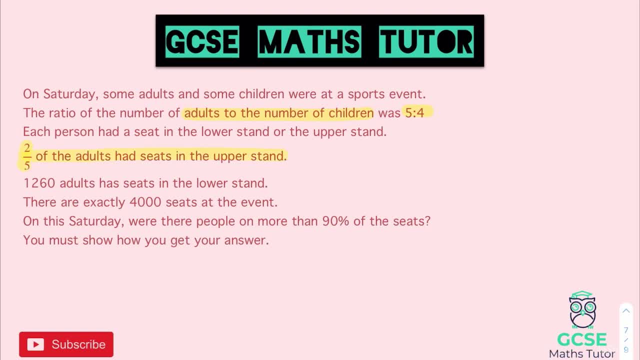 It says that two-fifths of the adults were in the upper stand, 1,260 adults were in the lower stand and there were 4,000 seats at the event, And it says were there more than 90% of those filled. 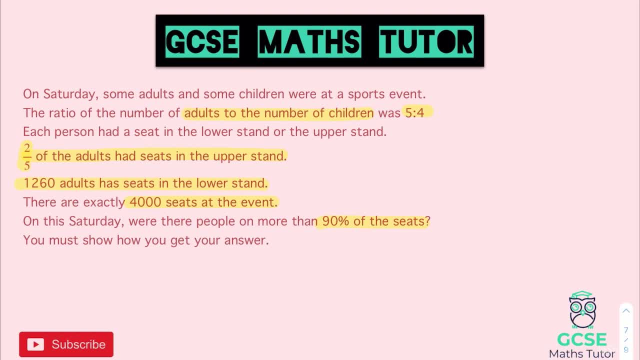 So, again, the first thing that I would work out here is 90% of 4,000.. And if you work out 10%, it comes out as 400, and you can actually just take that away from the 4,000, which gives you 3,600 seats that we're looking to see if they're filled. 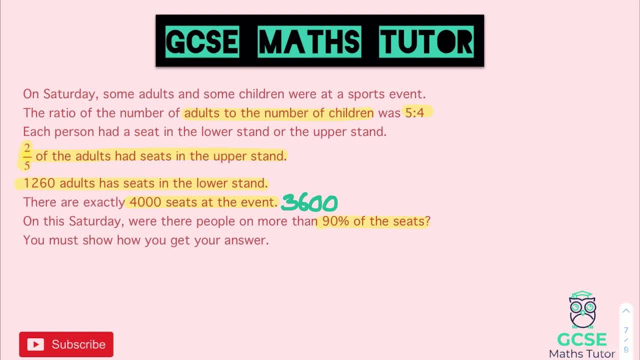 Or you could just do the 400 and times it by 9,, which again gives you the 3,600.. Moving on then. Now it says that two-fifths of the adults had seats in the upper stand. So if that is two-fifths, then the amount of adults in the lower stand must have been three-fifths. 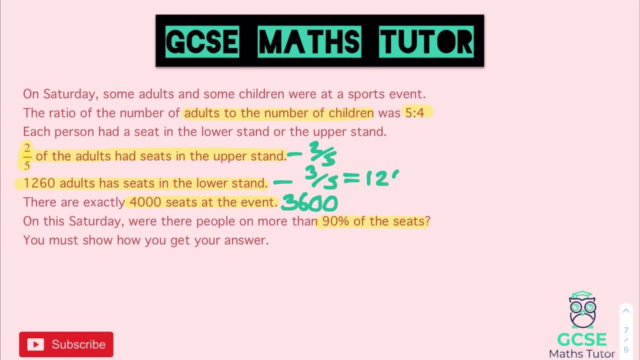 And we know that that three-fifths is equal. So that's equal to 1,260.. Now this is actually the one step in here which is a little bit harder than the last one, Because to get three-fifths to two-fifths that's a little bit more complicated. 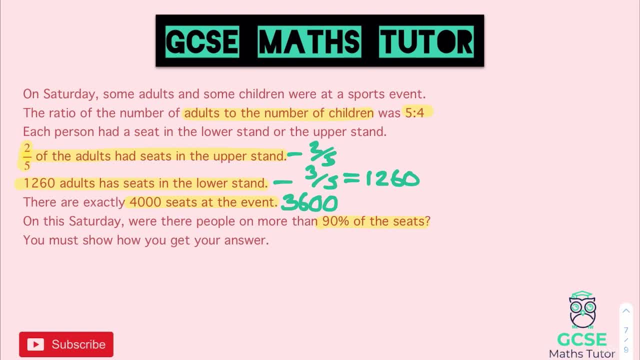 And in order to get that down to one-fifth, you would have to divide that by three, as that is currently three-fifths, And if we divide that by three, that would give us that one-fifth is going to be equal to 420.. 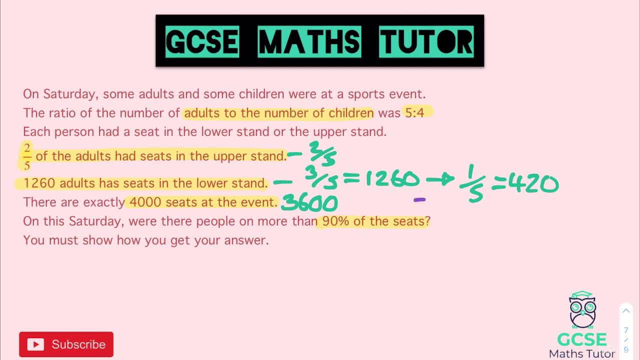 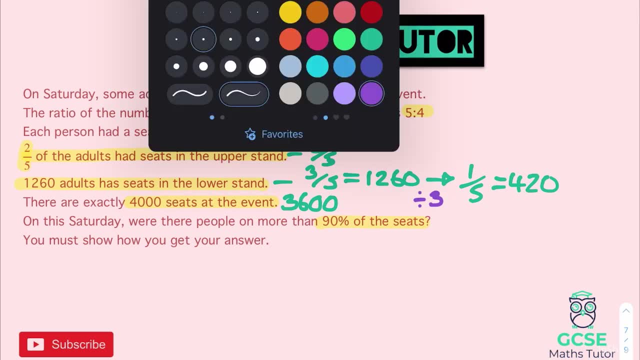 And again just writing the working out down there: we divided that by three. Remember, three-fifths divided by three would give us one-fifth. We can then multiply that by two and that would give us the amount for two-fifths. 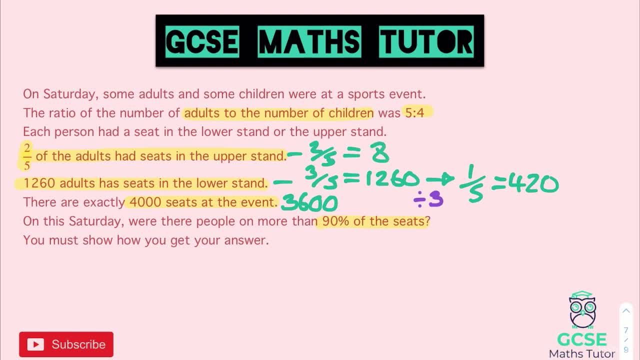 And if we multiply 420 by two, you get 840.. So that is the difficult part of the working out and how this was different to the last question. The rest of this is relatively similar. We're going to now find out how many children there are and we're going to re-share that into the ratio. 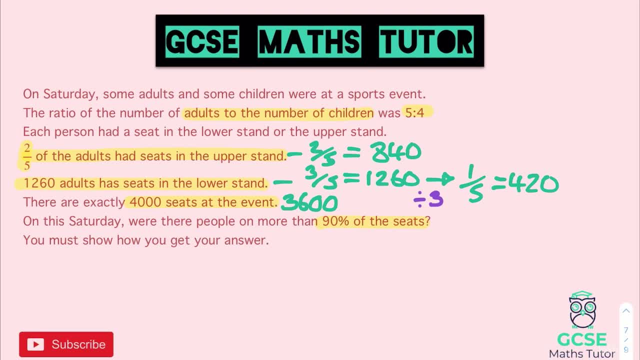 So that is the difficult part of the working out and how this was different to the last question. The rest of this is relatively similar. We're going to now find out how many children there are and we're going to re-share that into the ratio. 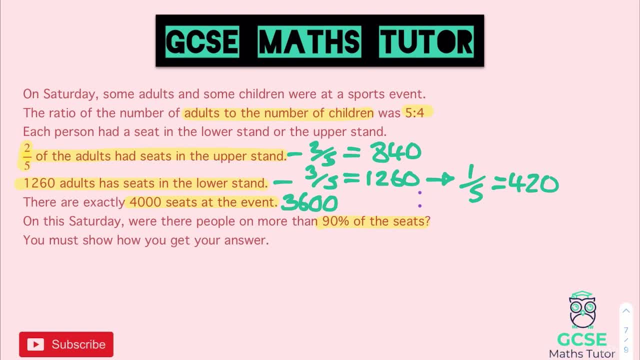 So if we get rid of a little bit of that working out there, let's just get rid of that, And what we're going to have a look at now is getting the total of the adults. So to get the total of the adults, 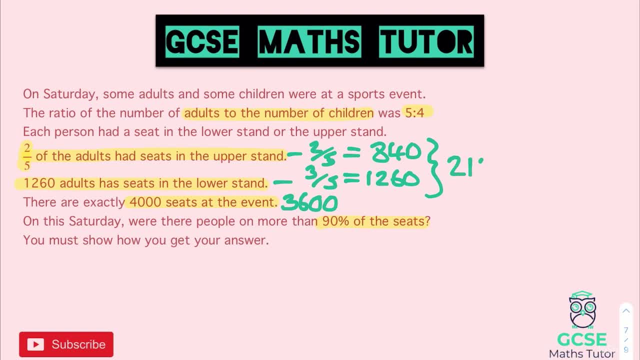 we'd add these two together and that gives you 2,100 adults. Now we can have a look at applying that to the ratio. In the question we're told that the ratio of adults to children is 5 to 4.. 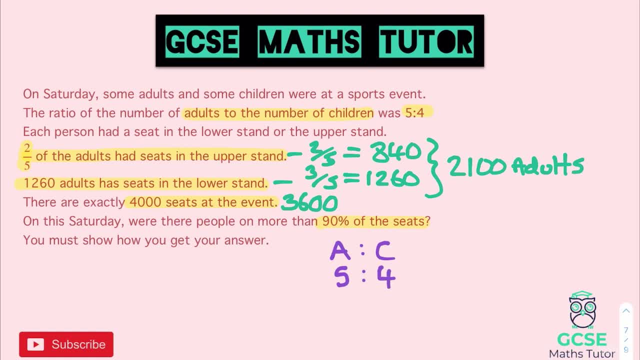 And we now know that there are 2,100 adults that are, in respect to that number, 5.. And we just have to figure out what you multiply by in order to get down to the 2,100.. And we'll do that. 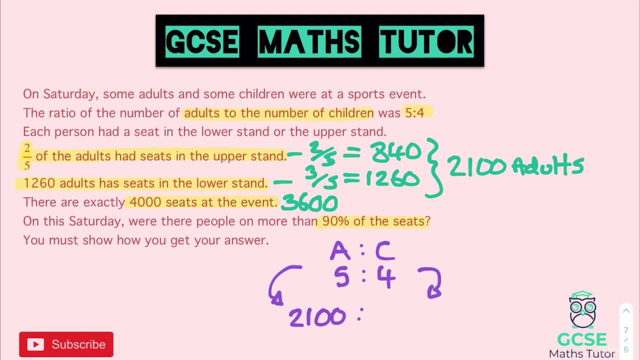 It's the same for the children. So to work that out, we need to do the 2,100 divided by 5.. Again, I will do this working out rather than rushing this last bit. But dividing that by 5 goes in four times. 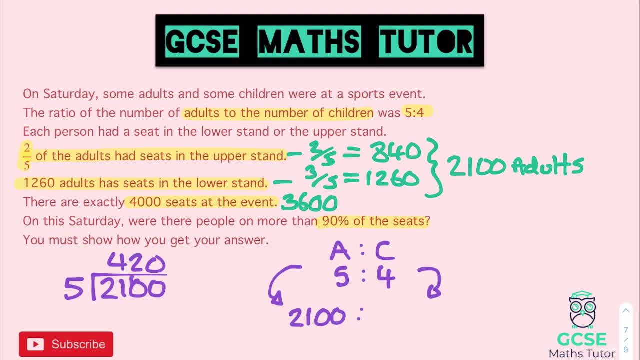 Carry the 1 to 0. So it's times 420.. So interesting that that came out as 420, because there was a 420 earlier on in the question but not necessarily related to one another here. So there we go, Timesing each of these by 420. 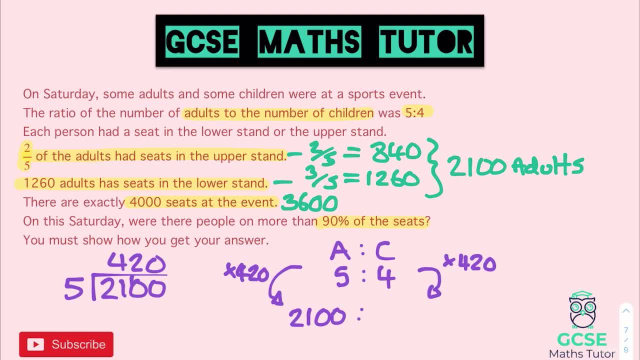 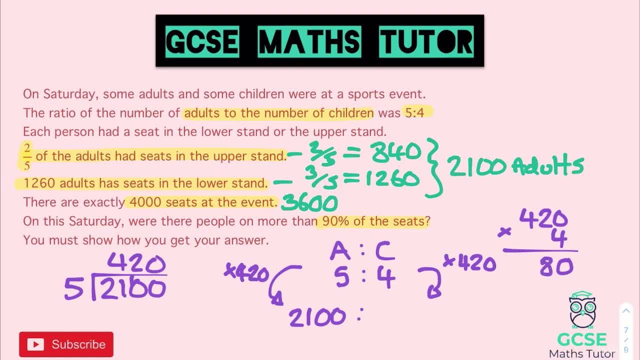 4 times 420.. 4 times 0 is 0.. 4 times 2 is 8.. And 4 times 4 is 16.. So we have 1,680 children. OK, so on to the last step then. 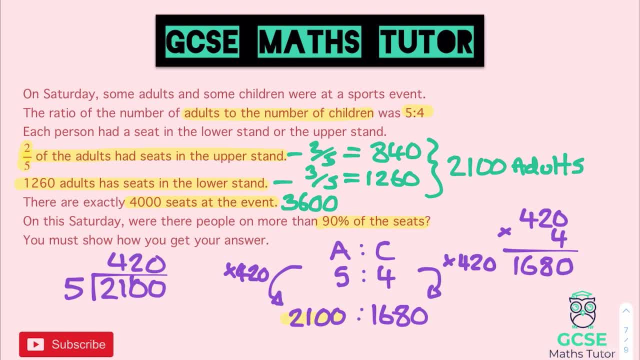 We now know how many adults there were: 2,100.. How many children there were: 1,680.. In order to get the total, we just have to add those two together and compare it to that: 90%, So 2,100.. 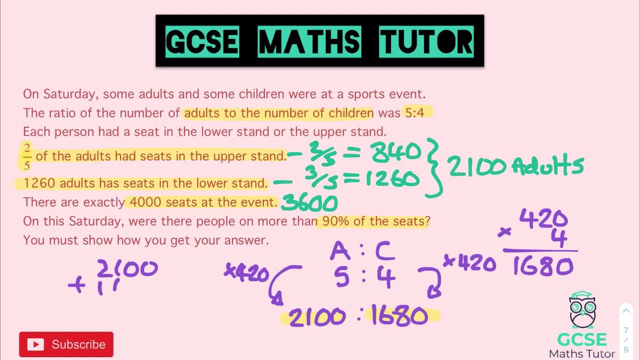 And again, don't forget, it says you must show how you got your answer. So even if you can see if that's under or over, you still need to make sure you write this down. So 0,, 8,, 7,, 3.. 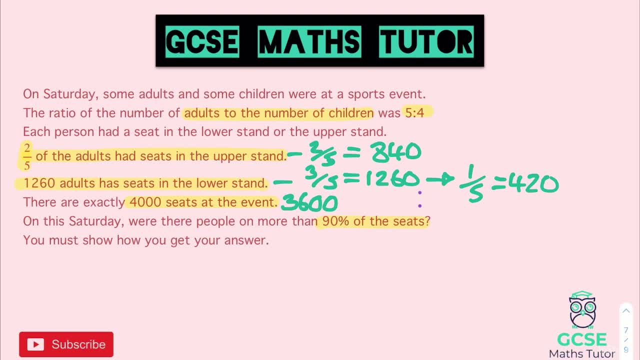 So if we get rid of a little bit of that working out there, let's just get rid of that, And what we're going to have a look at now is getting the total of the adults. So to get the total of the adults, we'd add these two together and that gives you 2,100 adults. 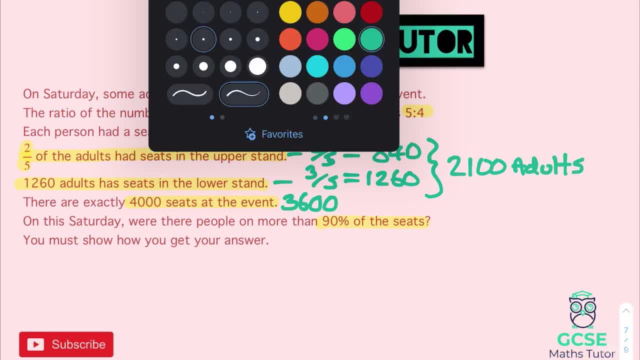 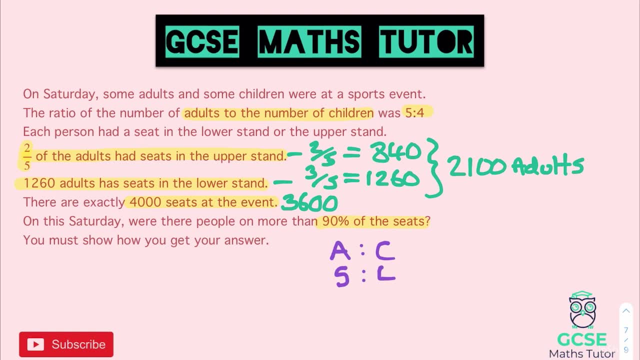 Now we can have a look at applying that to the ratio. In the question we're told that the ratio of adults to children is 5 to 4. And we now know that there are 2,100 adults that are, in respect to that number, 5.. 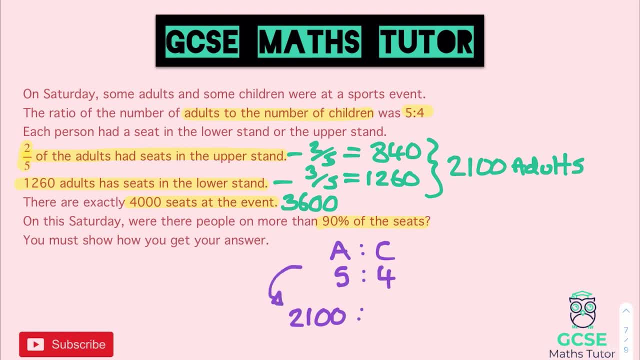 And we just have to figure out what you mean: Multiply by in order to get down to the 2,100.. And we'll do that. It's the same for the children. So to work that out, we need to do the 2,100 divided by 5.. 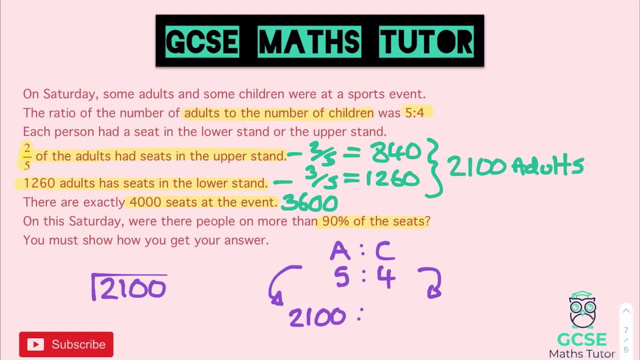 Again, I will do this working out rather than rushing this last bit. But dividing that by 5 goes in four times Carry the 1 to 0. So it's times 420.. So interesting that that came out as 420, because there was a 420 earlier on in the question. 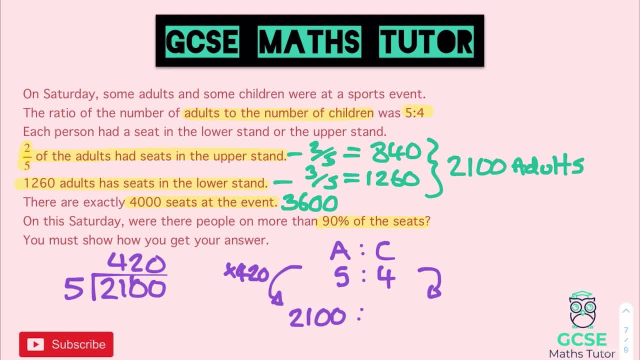 But not necessarily related. I'll just do one another here. So there we go, timesing each of these by 420.. So 4 times 420. And again, you can just work that out to the side. Well done, if you're sitting at this point thinking you've already got this. 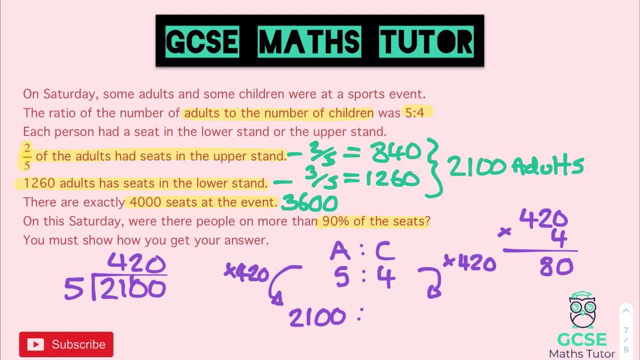 4 times 0 is 0.. 4 times 2 is 8.. And 4 times 4 is 16.. So we have 1,680 children. Okay, so on to the last step. then We now know how many adults there were: 2,100.. 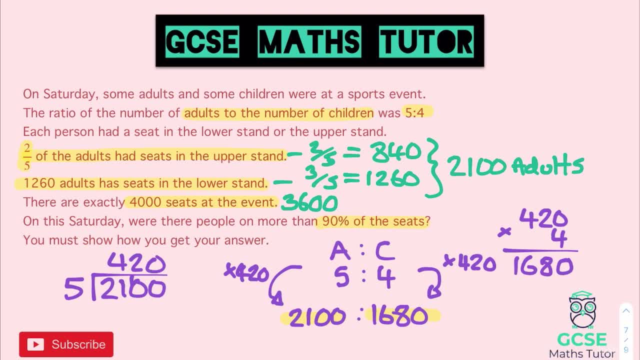 How many children? there were 1,680.. In order to get the total, we just have to add those two together and compare it to that: 90%, So 2,100.. And again, don't forget, it says you must show how you got your answer. 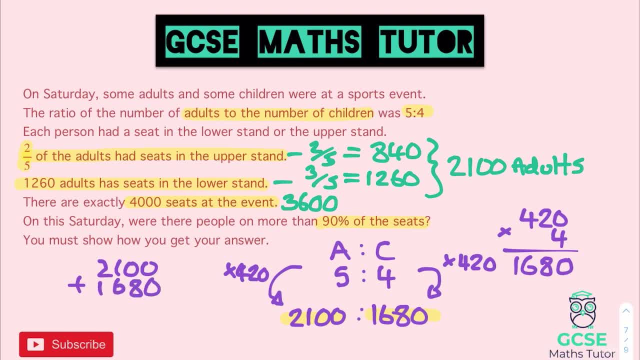 So even if you can see if that's under or over, you still need to make sure you write this down. So 0, 8, 7, 3.. So 3,780.. And that is more than the 3,600.